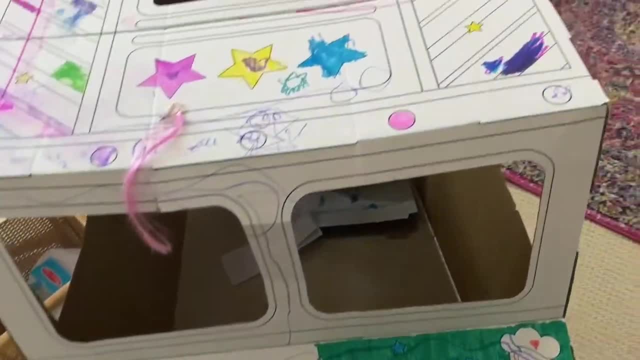 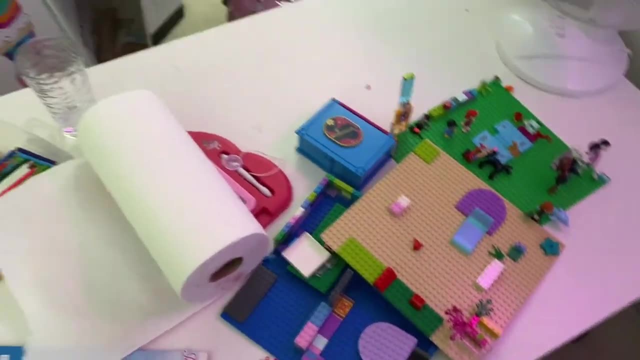 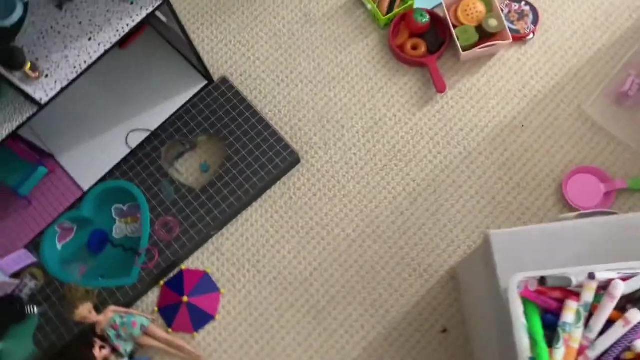 letting them tidy their own room, but it hasn't been deep cleaned all summer School starts next week, so it's the perfect time to reset. My goal for these upcoming videos is to get back to basics, and what that means is really focusing on deep cleaning, decluttering and organizing the entire. 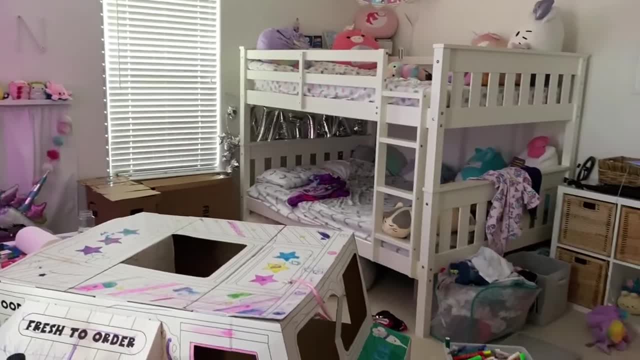 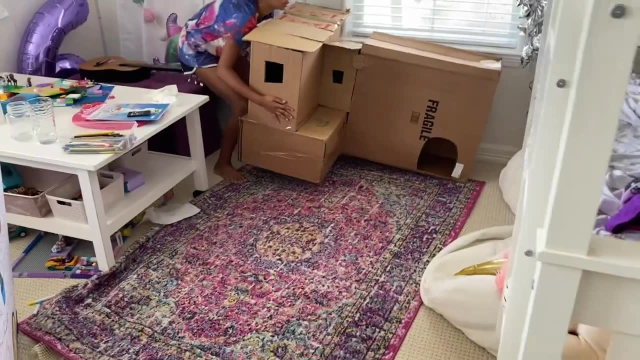 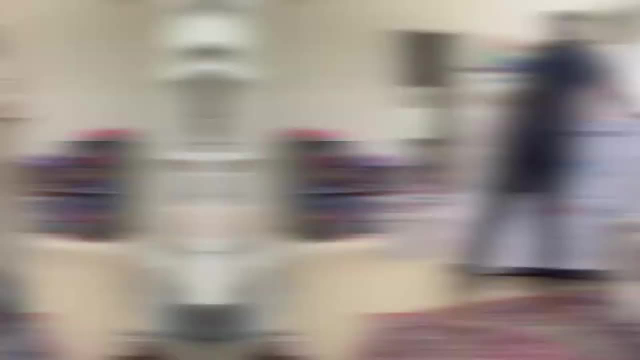 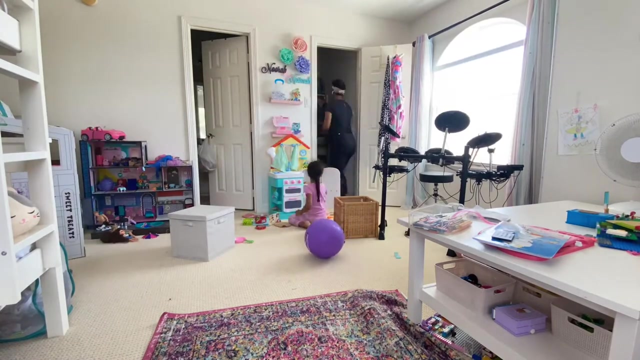 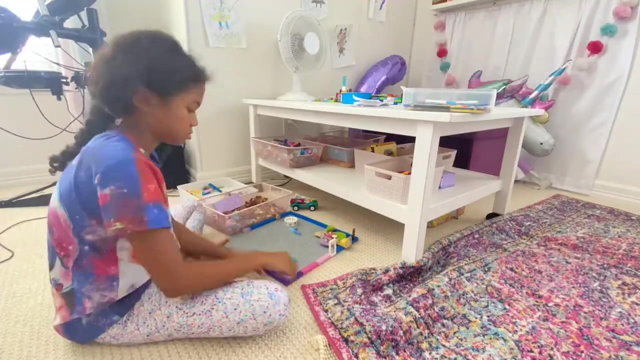 house, one room at a time. In today's video we're going to be decluttering and organizing the girls entire room. Let's go Have fun watching. We used to ace All I, you and me. We used to ace All I, you and me. 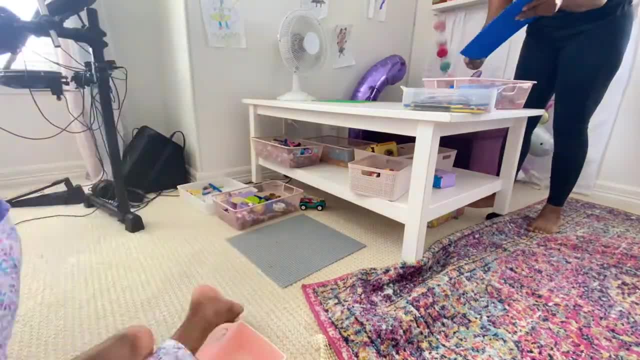 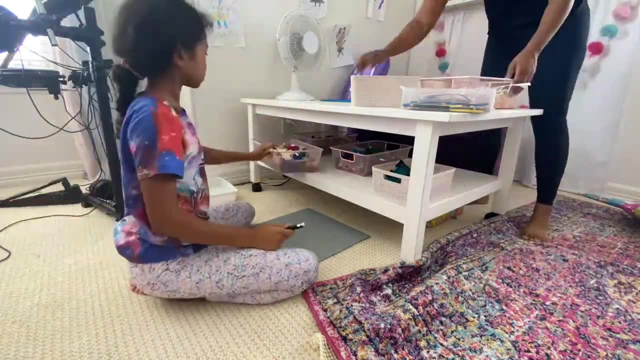 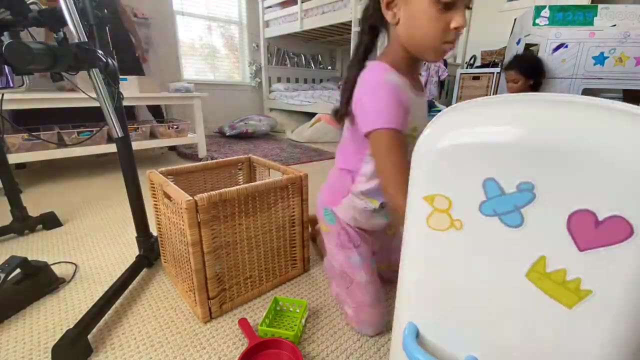 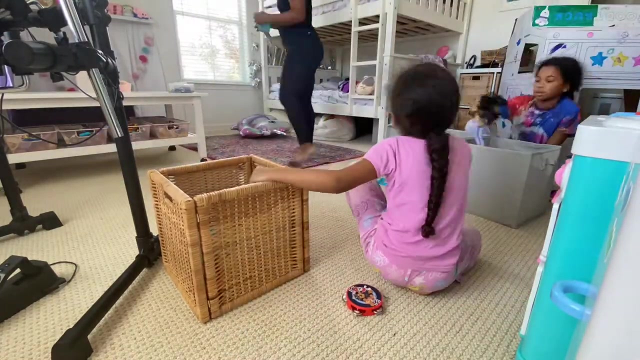 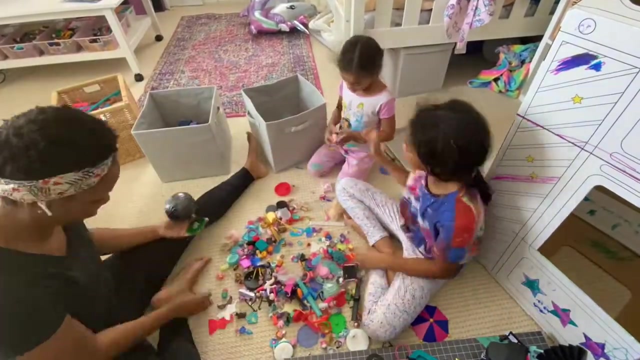 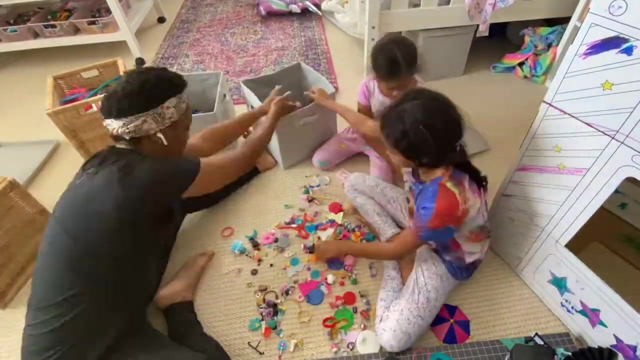 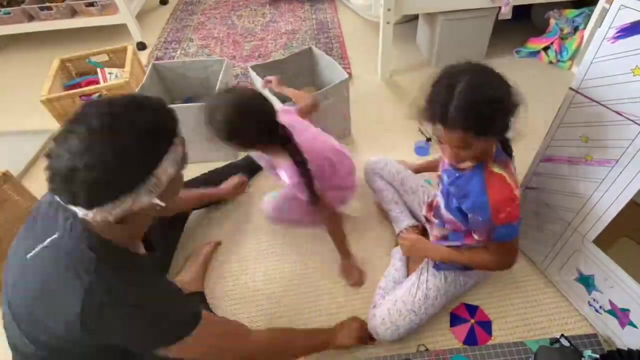 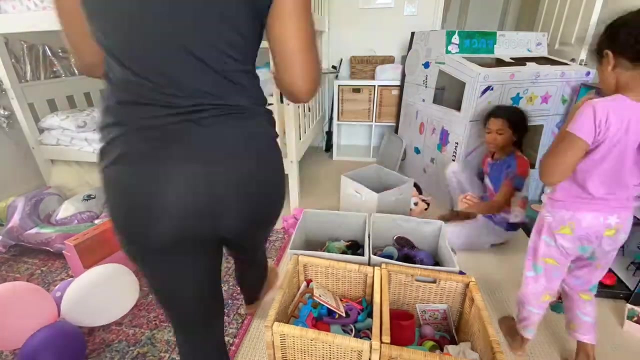 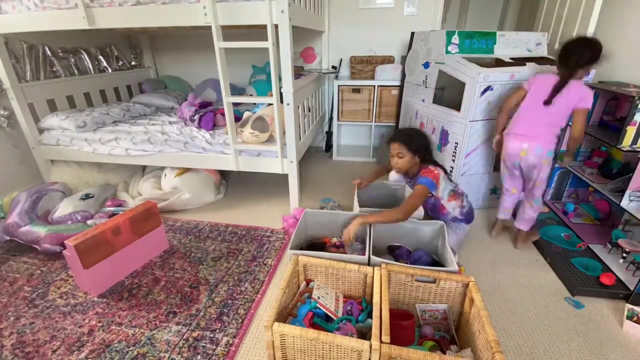 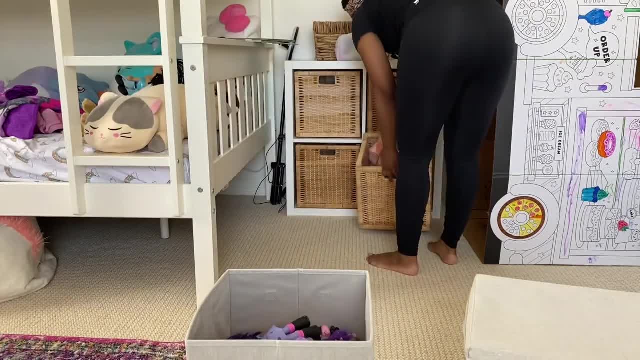 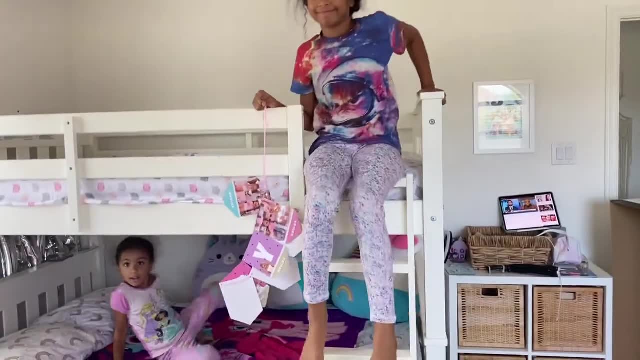 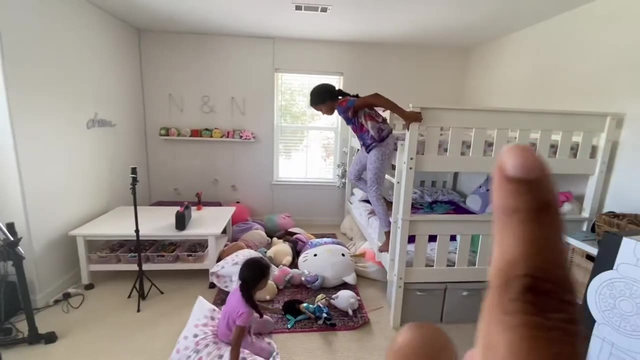 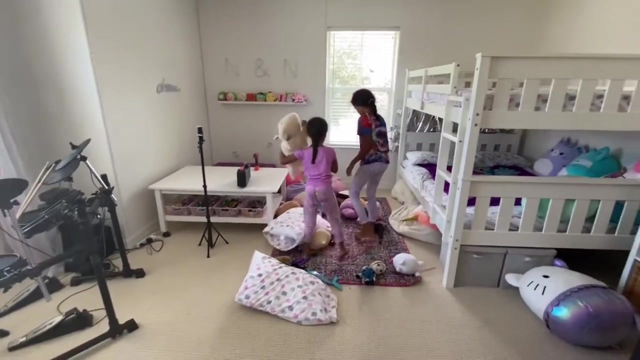 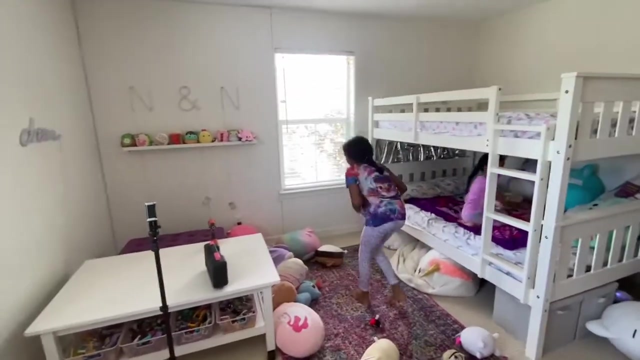 We used to ace All I, you and me. My big girl is finally getting separate bed and she's on the floor now. We're going to put Noura's bed on this side after we separate the bunk beds. So we're going to do a little bit of rearrangement of their room so that their beds are side. 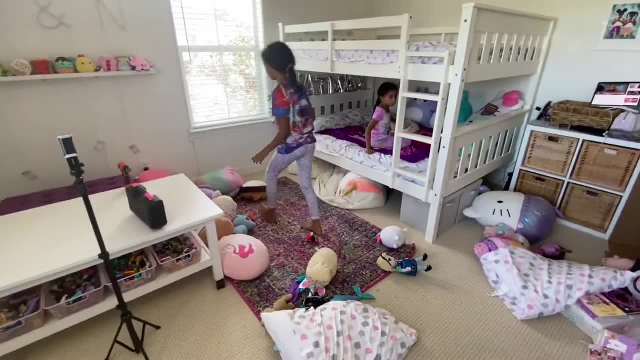 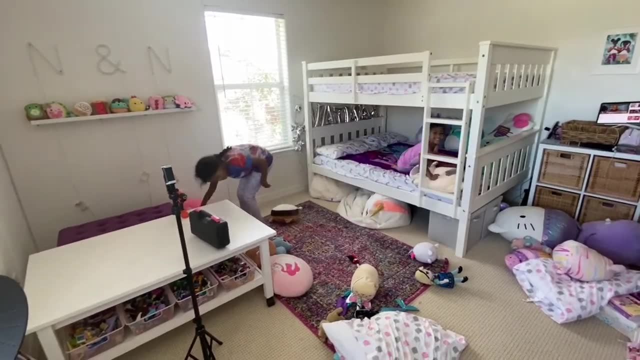 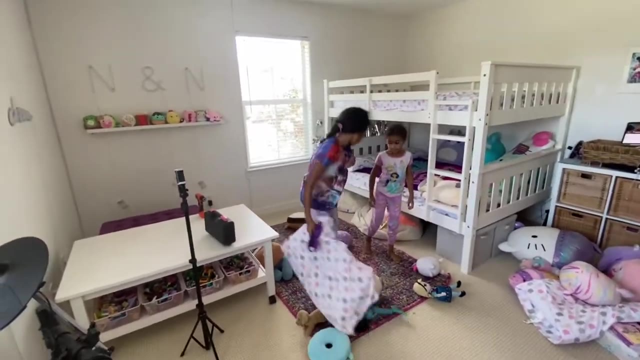 by side: Noura's taking everything off her bed. Naima's supposed to be making her bed. She's taking forever. So I think this is going to turn into two days of deep cleaning the girls' room because I want the girls involved and helping. 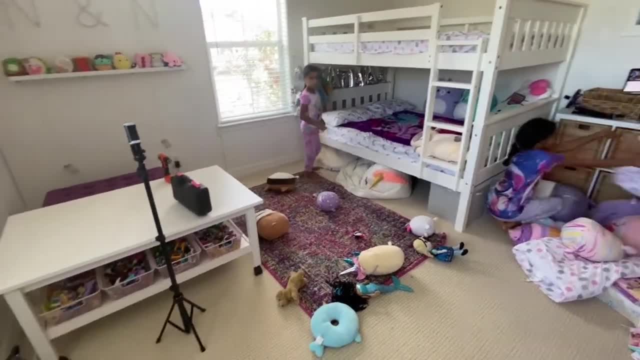 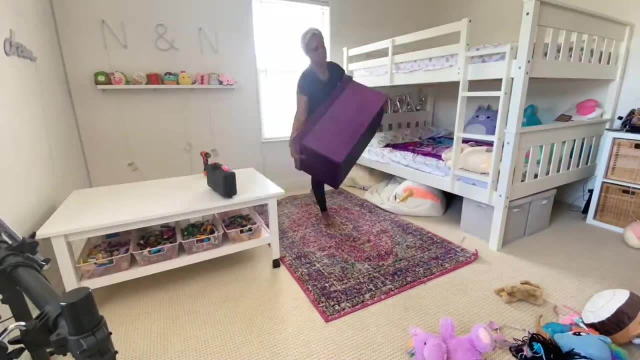 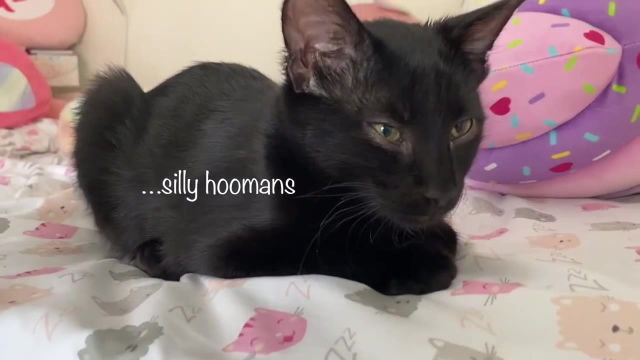 We also need to do the closet and we also need to do the bathroom, But for now we're going to do the main part of the room first. I want to be there and baby dance the night away. I let my head down if I want. 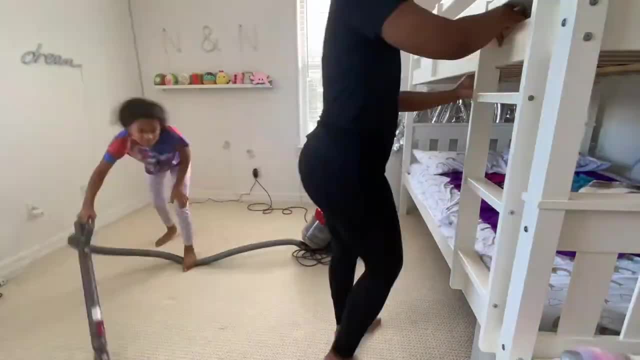 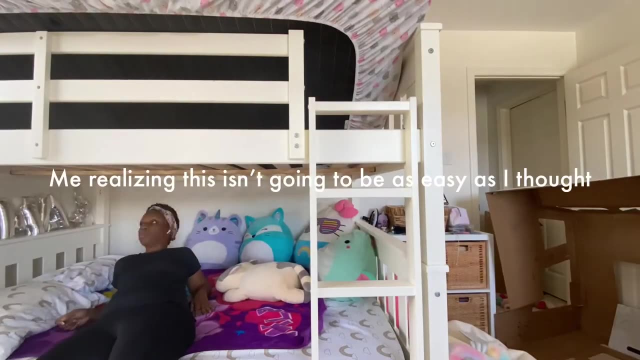 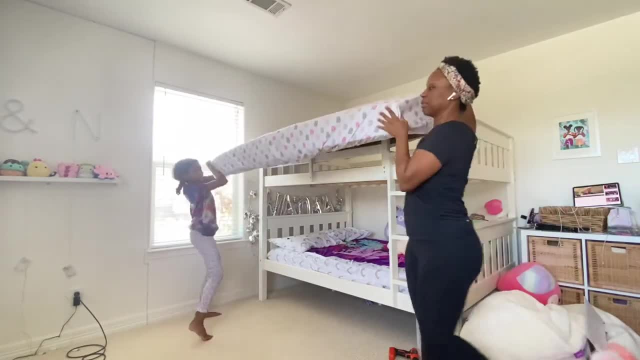 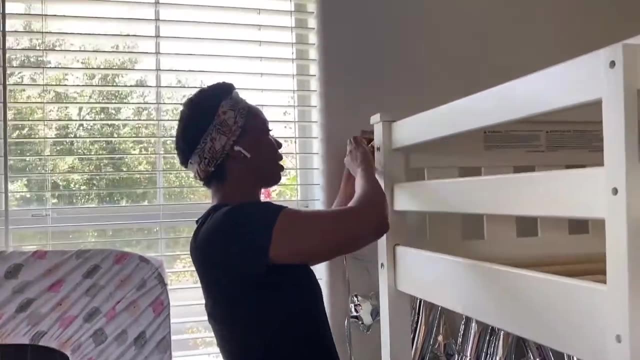 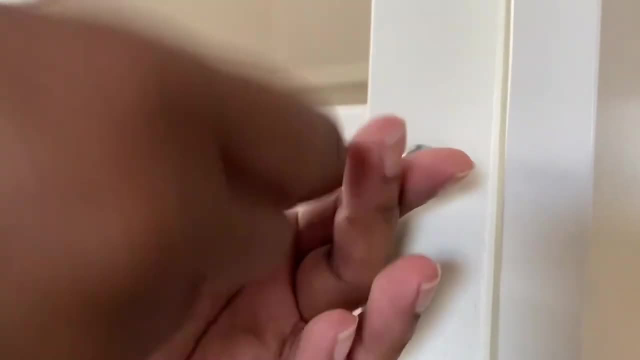 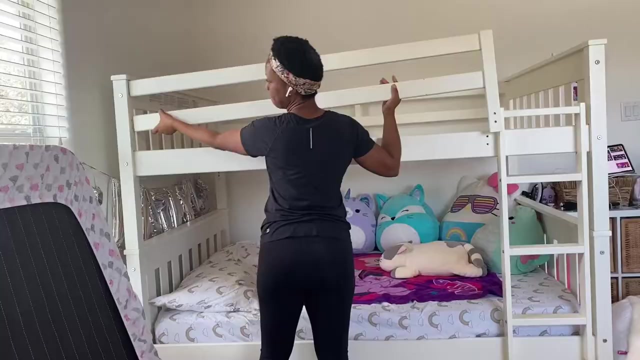 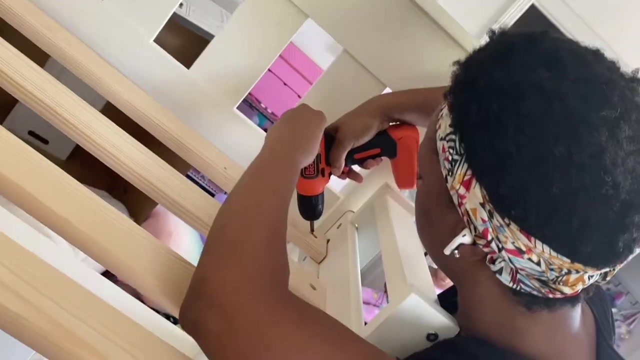 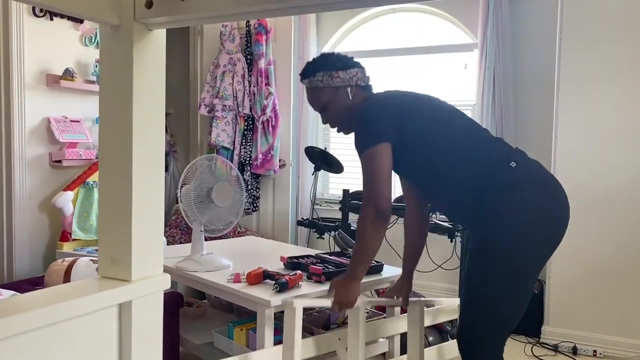 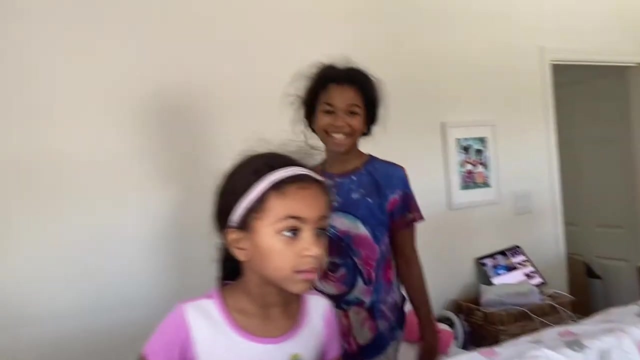 be Noura's bed. I want to be silly baby. Dance the night away. I'll kick my shoes off. If you can't do better, I dare you to be wilder. I want to be silly baby. okay, with my husband's help, I was able to take off the top bunk and it looks so. 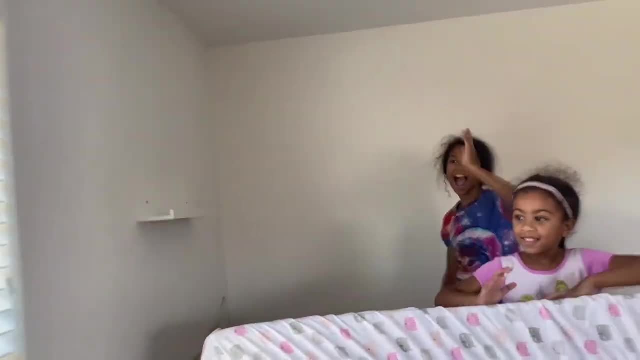 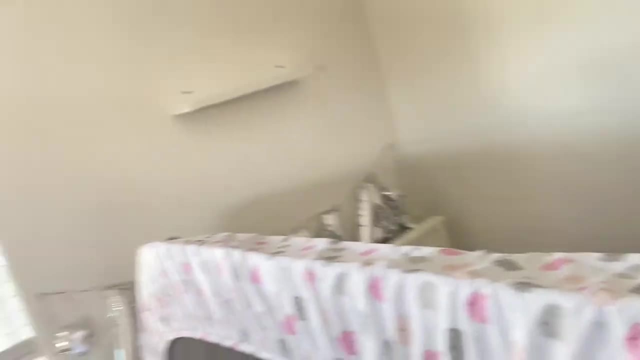 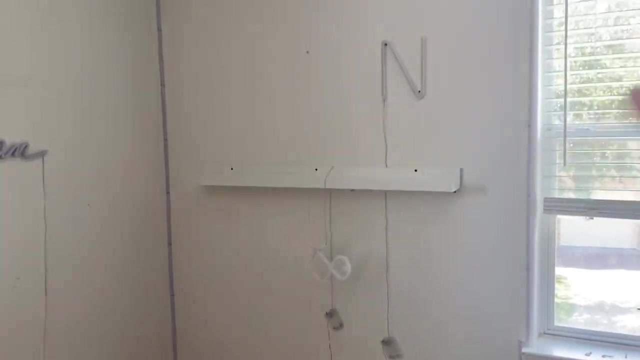 much brighter. I didn't. I took for granted how much light they get in here, but this area of the room is a lot brighter without the top bunk. so right now, while I have the chance, before I put the bed back over here, I am moving things around. 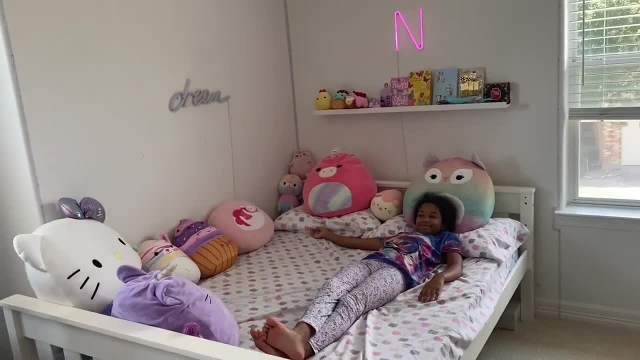 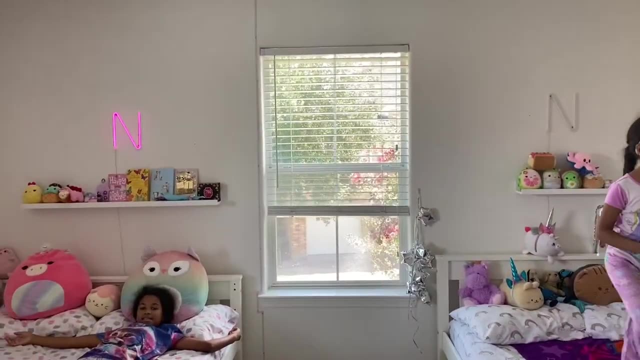 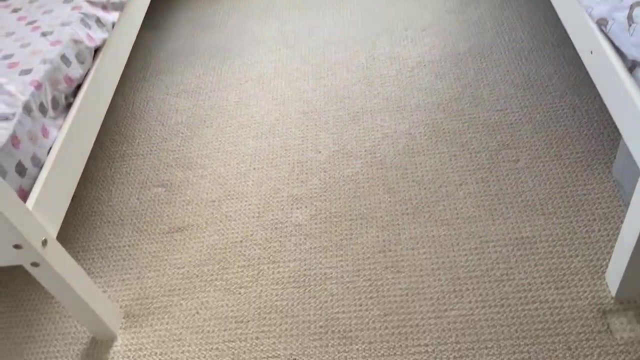 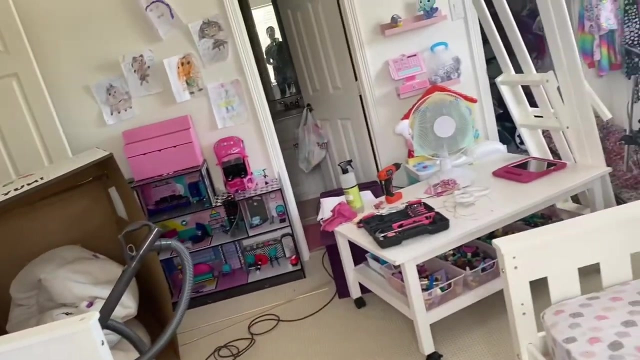 all right. so Noora's bed is moved and they are both making their beds. I move the shelves down, I move one end to the other side. I am just vacuuming. I'm gonna put the rug back here. the rest of the room is kind of a mess, hi y'all. um, and so what I thought I was going to do is I'm going to put the rug back here. 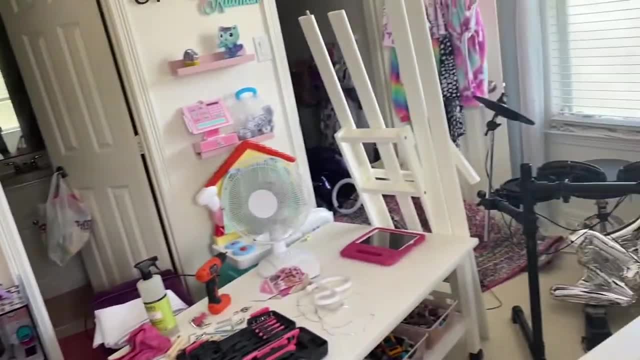 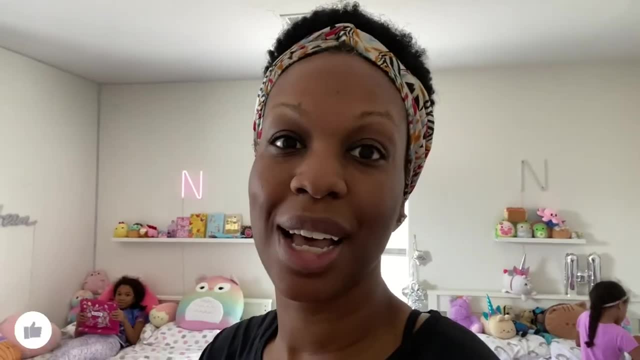 as I am gonna put them back in their closet. but before I done that, I want to tell you that one, which is the second bed, bed which I like to do in a day. I'm pretty sure I'm going to need that second day because I still want to. 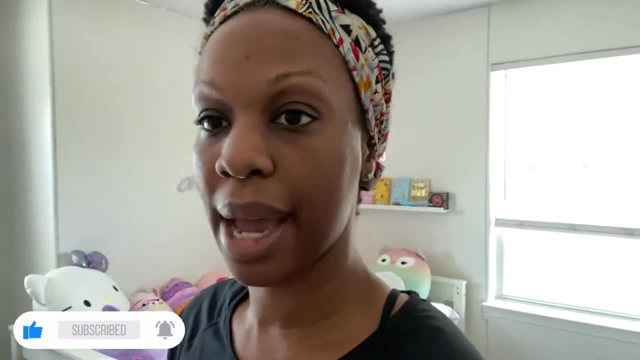 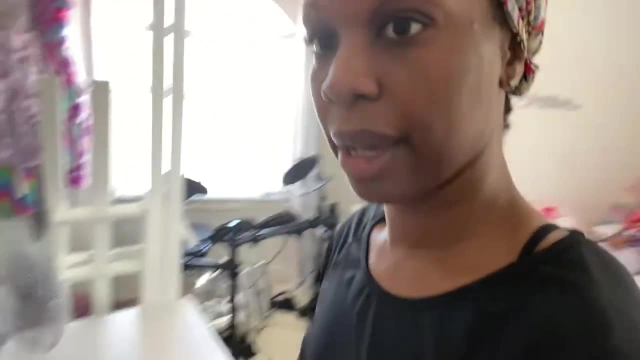 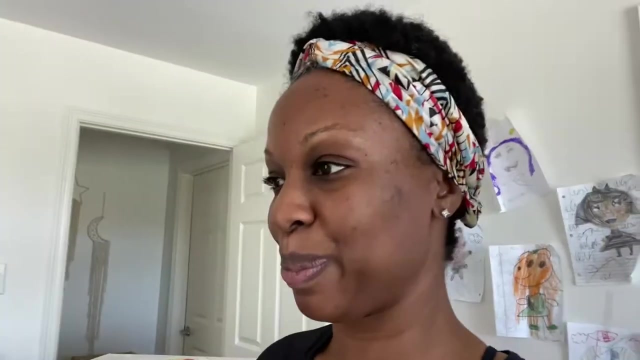 tackle their closet and their bathroom. I hope you guys like this video and find some inspiration, but for now we are going to get back to kind of rearranging things and I'm trying to figure out where I'm gonna put their Lego table, I'm sure, but we're gonna get it together, but for now it's looking pretty good. 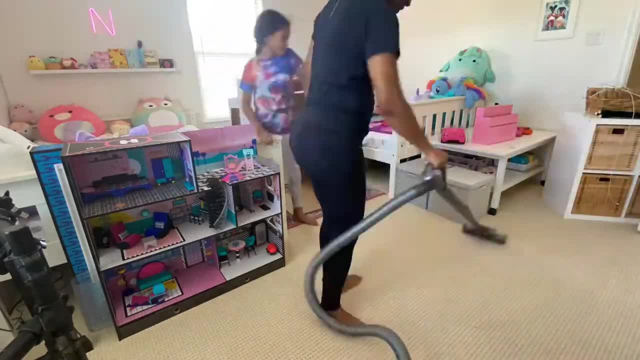 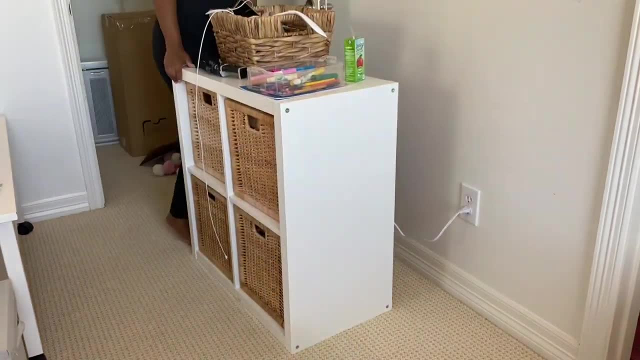 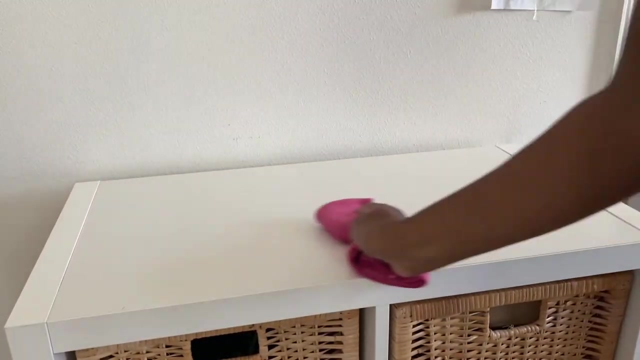 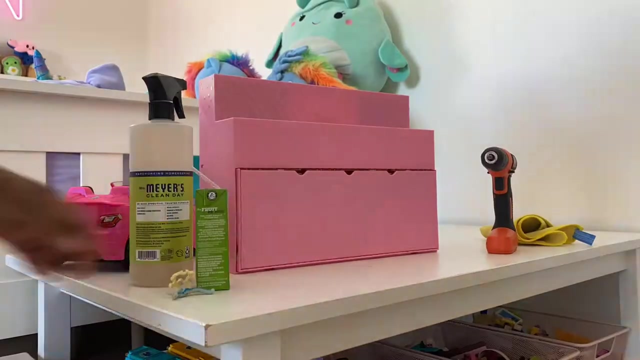 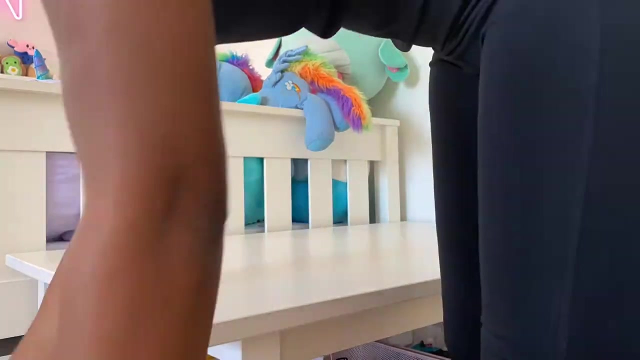 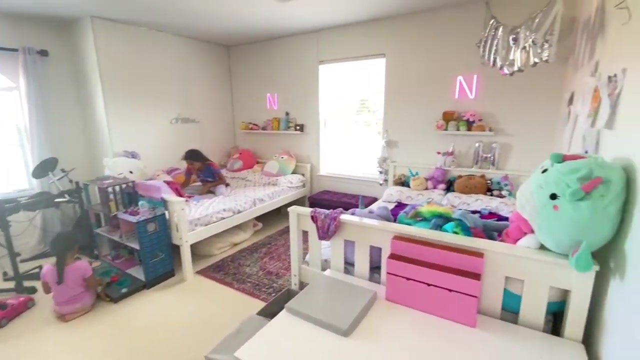 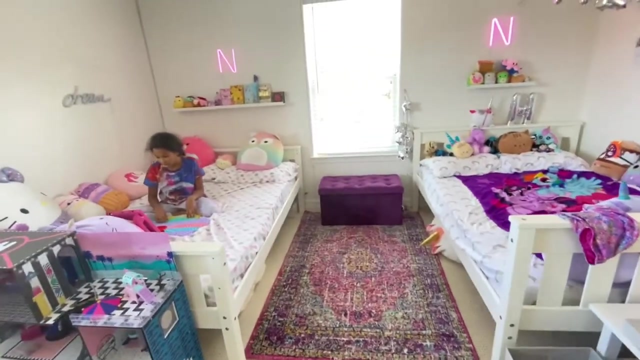 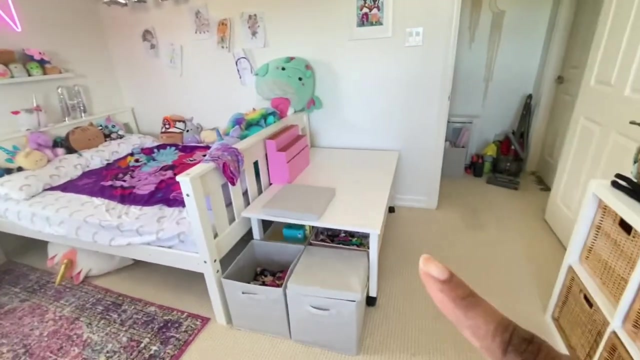 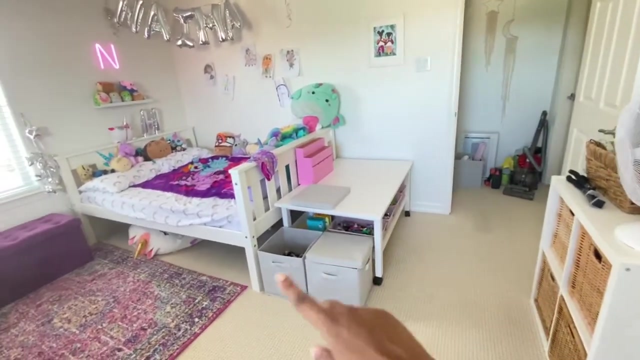 You All right. here's the room progress so far. The bunk beds are now two full beds. We still have the rug and the Stool, no storage ottoman. We move the Lego table in front of the little ones bed. I'm thinking I might want to get some under bed. 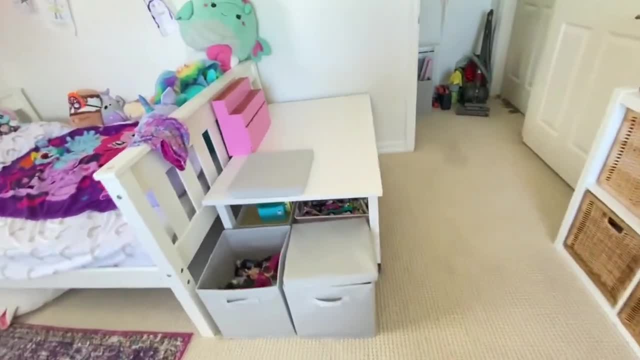 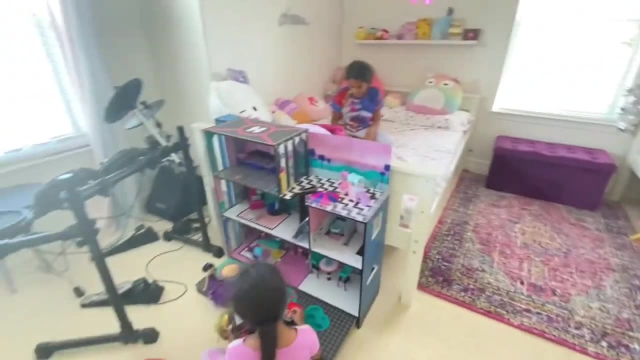 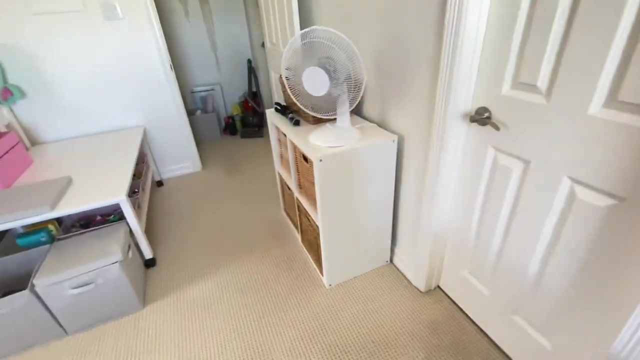 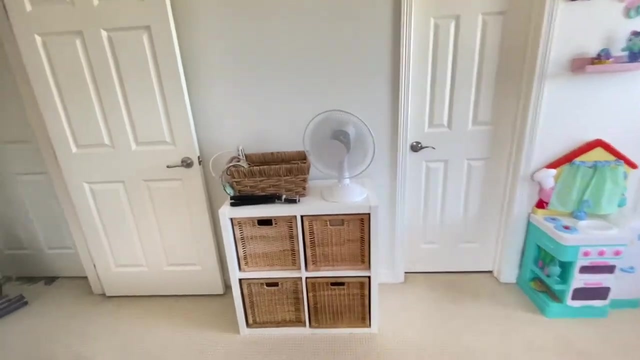 Storage so that we can move these two Bins under her bed. and then we move the lol house in front of the big ones bed and We put the, The other toys, the other chest of toys, on back on this wall And this is their electronics basket. So we put all their electronics- They're charging here. 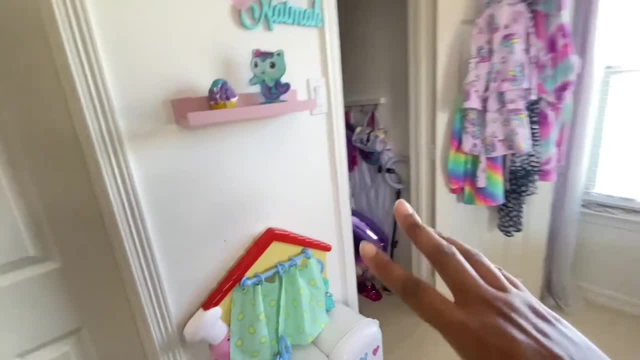 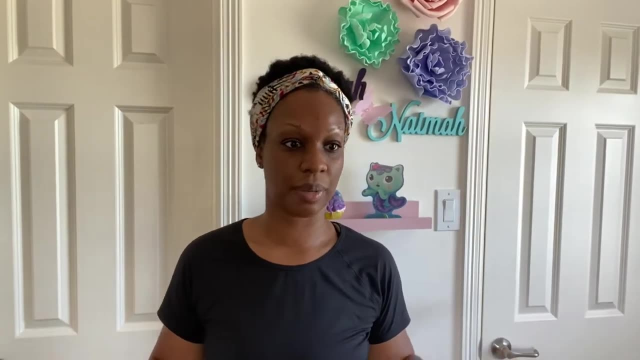 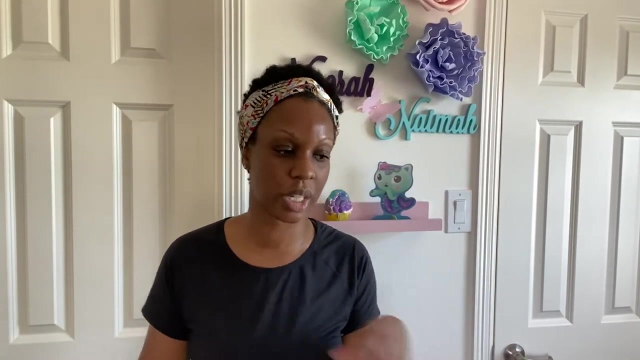 and I think I took one shelf down so that we can put Peppa Pig's kitchen Flush against the wall. All right, guys, so we've got a lot accomplished today. We got the bed separated, we rearrange their toys and storage furniture. I am pooped also have to take the little ones to swim practice. 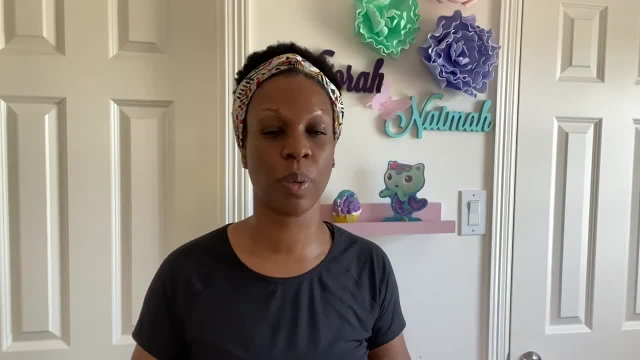 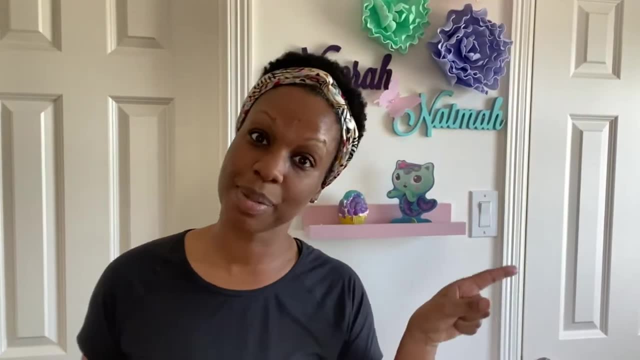 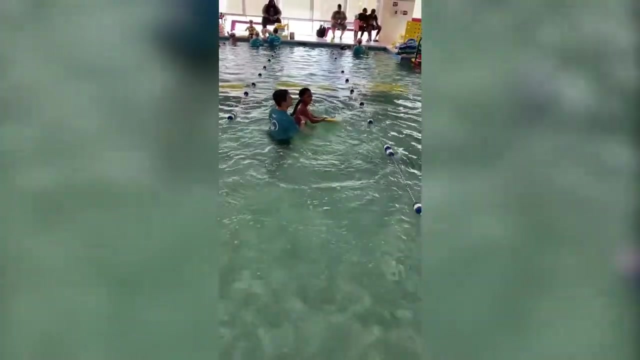 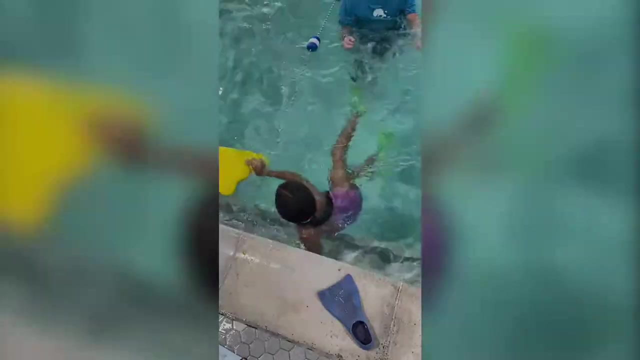 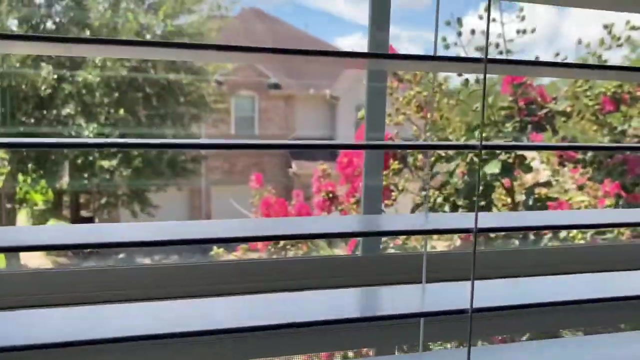 so we're gonna have to carry this over to a day to where we're going to tackle the closet and Clean the bathroom. So that's it for today. See you guys tomorrow. Bye, Hey guys, all right, it's day two of the deep cleaning. 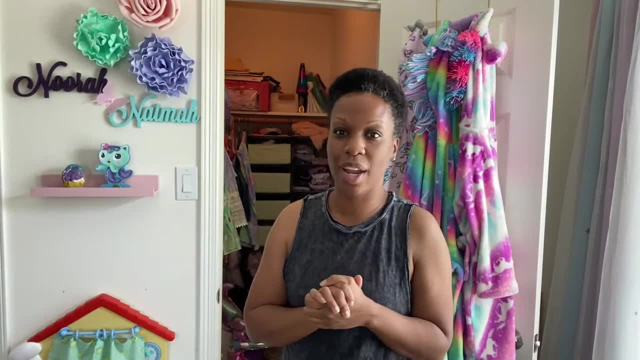 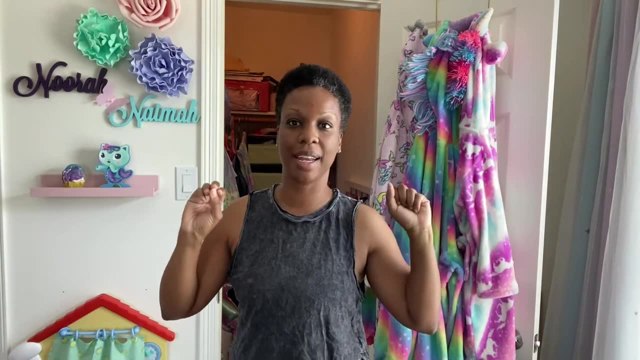 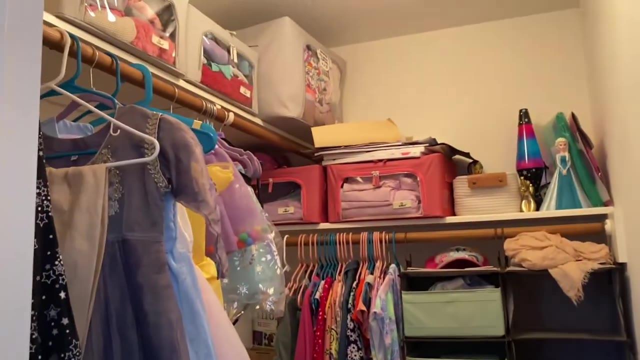 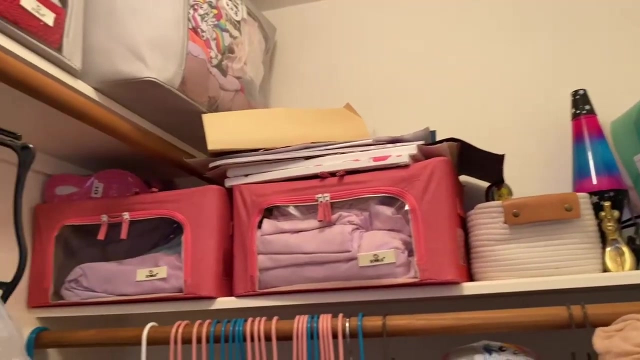 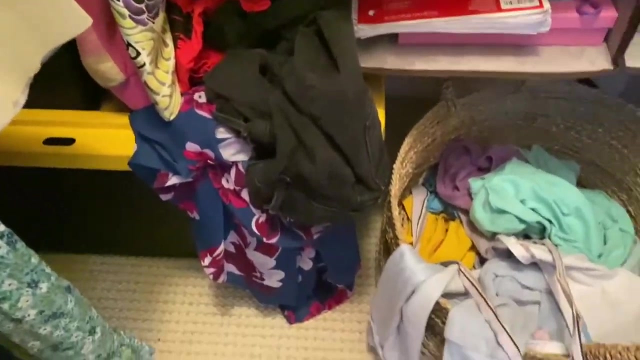 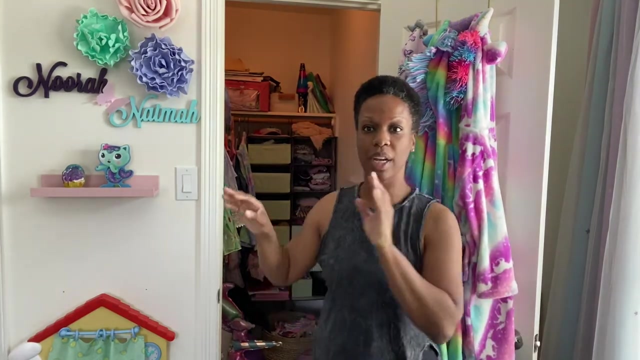 of my girls room. if you guys remember, yesterday we Separated the bunk beds, We move some things around and Now today we are tackling their closet. So my goal for their closet is to take out anything that they don't need, Organize the things that are there and just get it cleaned up and streamlined for when they start school next week. right, Let's go. 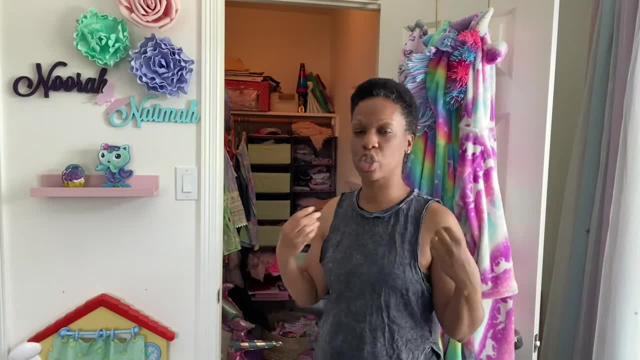 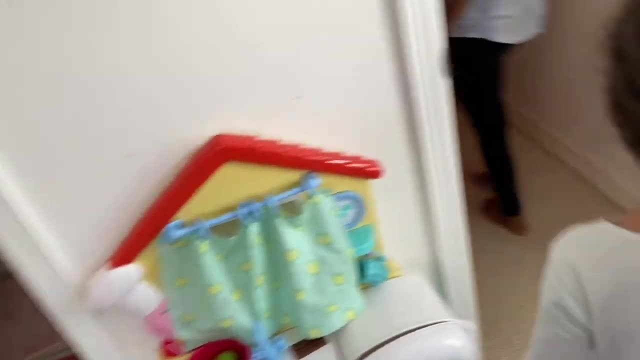 So my goal for their closet is to take out anything that they don't need, Organize the things that are there and just get it cleaned up and streamline for when they start school next week. All right, let's go, We're gonna take out everything except for the clothes and kind of go through. 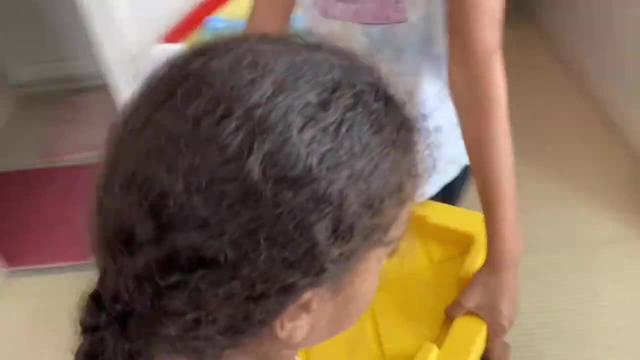 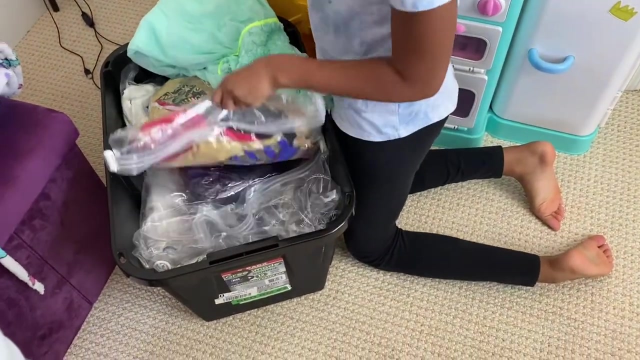 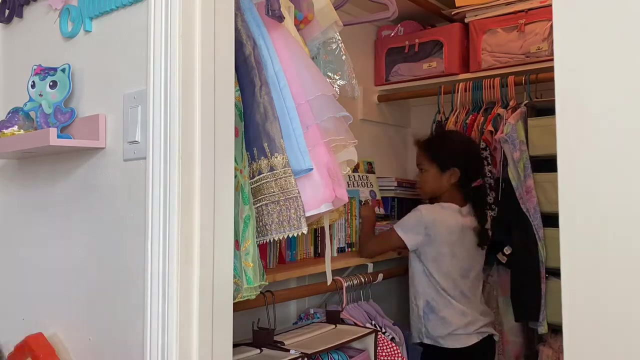 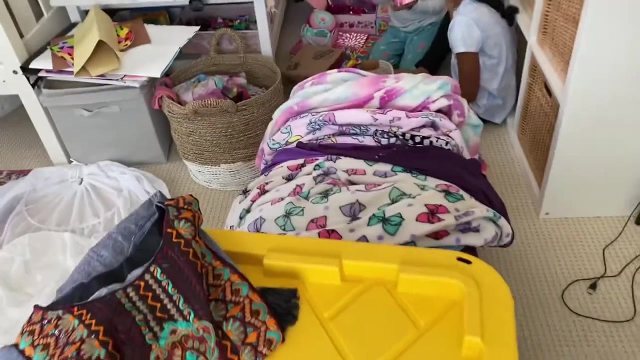 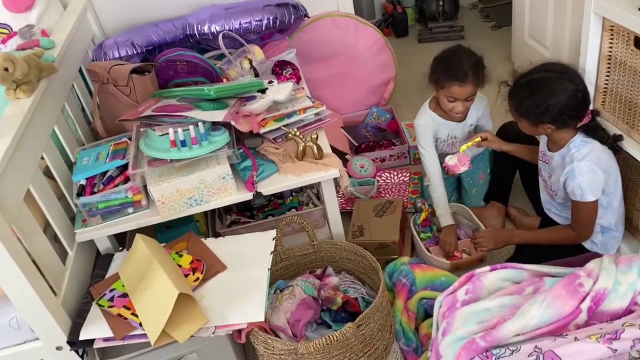 Go through everything and declutter What's in here: Our books, Old books maybe, eh, dresses. This is the progress of taking all the things out of the closet except for clothes, and we've got quite a bit of stuff to go through. and, guys, I love that when I do some housework with our kids. 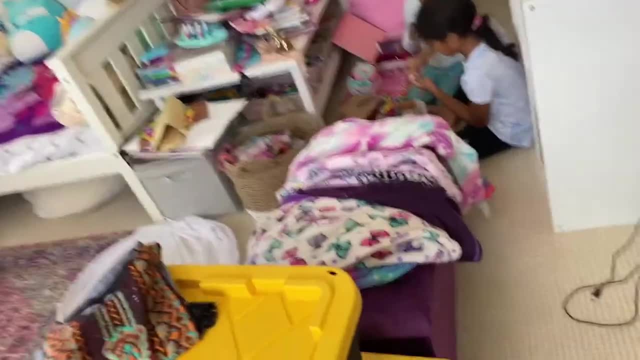 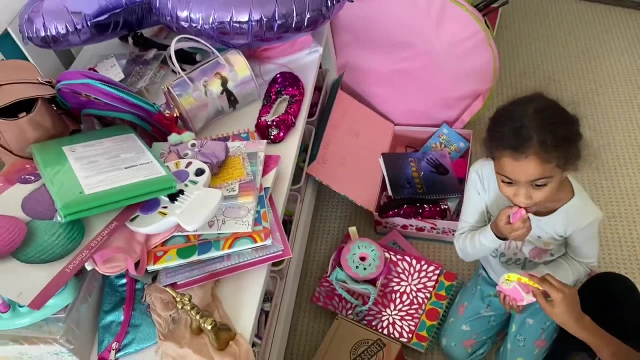 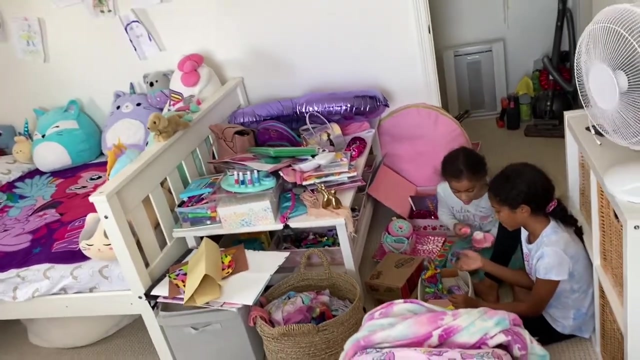 through and declutter. the girls are going through stuff that they totally forgot that they had, that they don't ever play with, so we're gonna have a hard time getting rid of some stuff i see, but we're gonna go ahead and declutter these items before we start um going through the clothes. 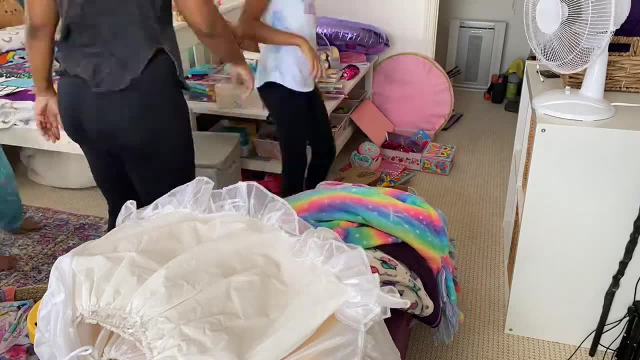 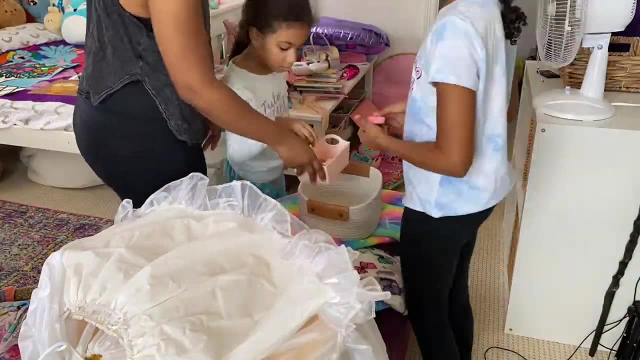 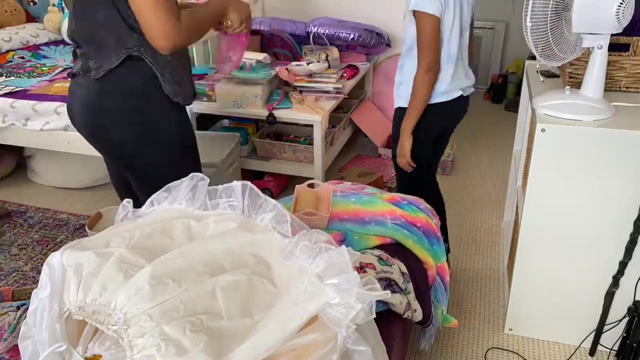 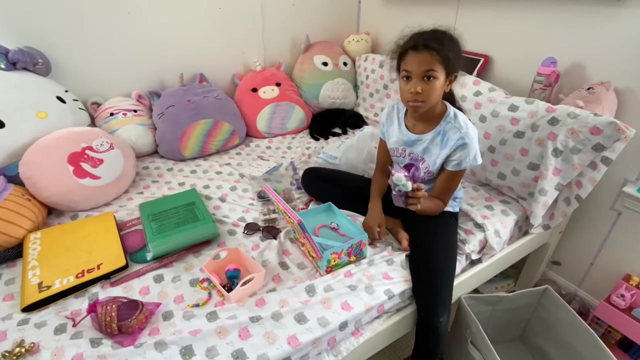 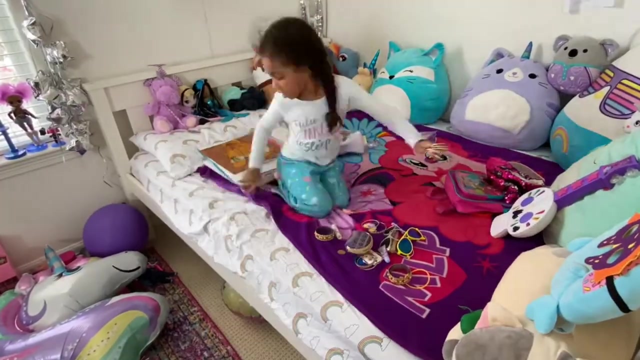 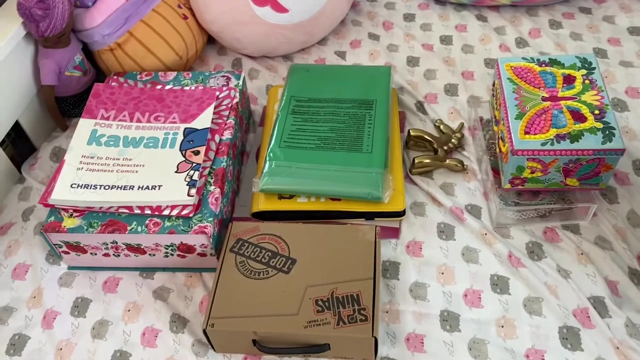 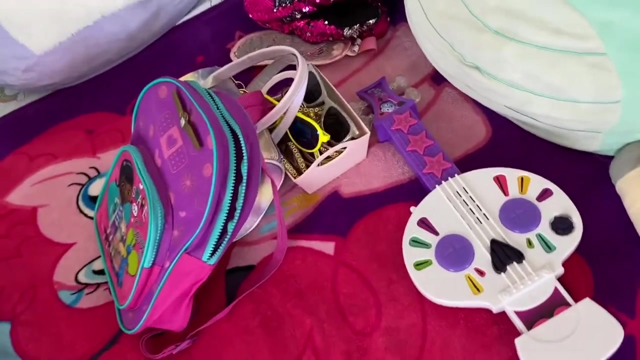 so, all right, guys, time for an update. we're making progress, even though it's slow, but the girls went through their things and this is what the big one is keeping. and then, um, we found a few things for the little one to keep. we got some artwork that we might end up framing, um, and 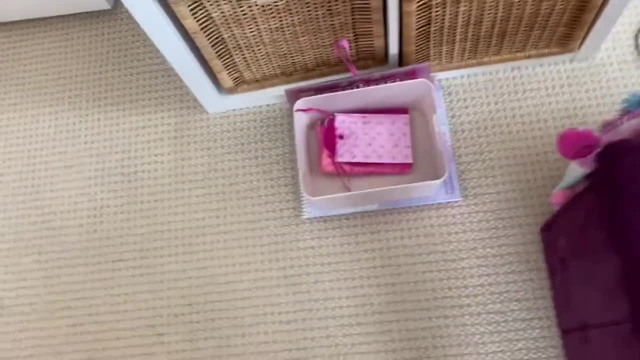 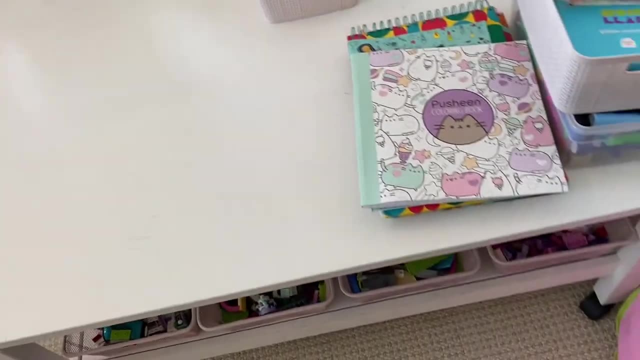 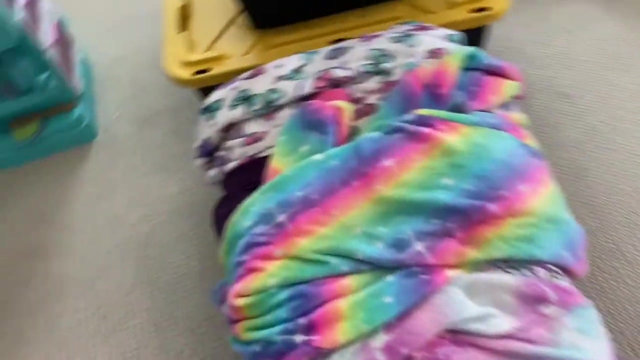 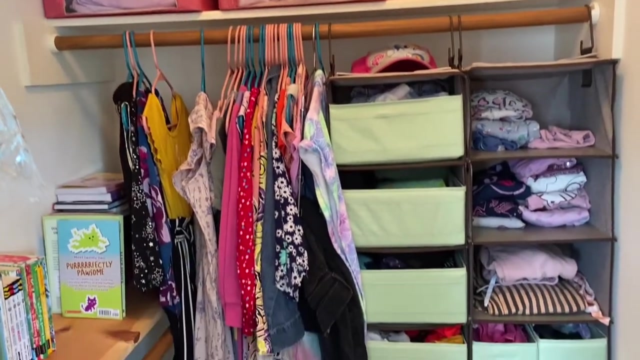 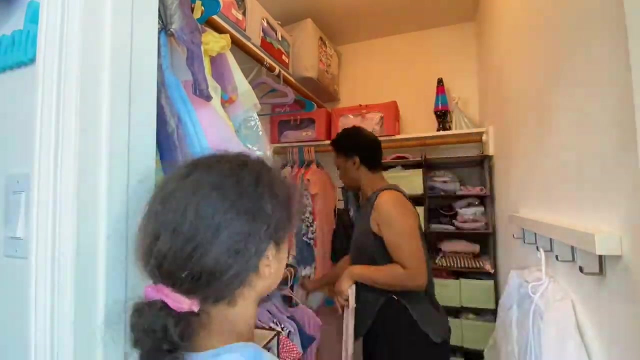 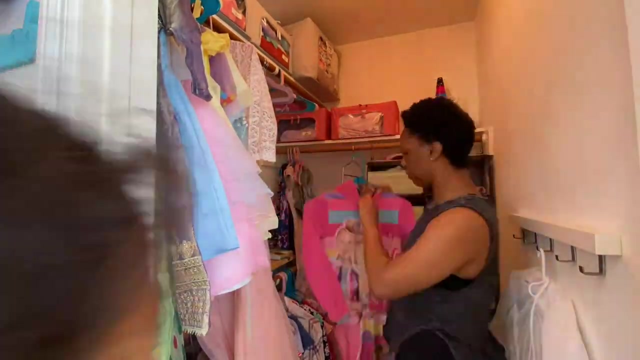 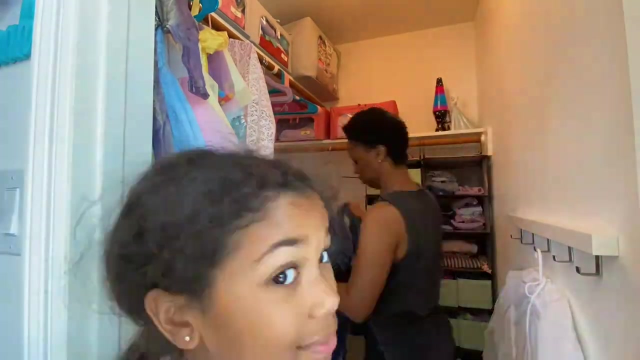 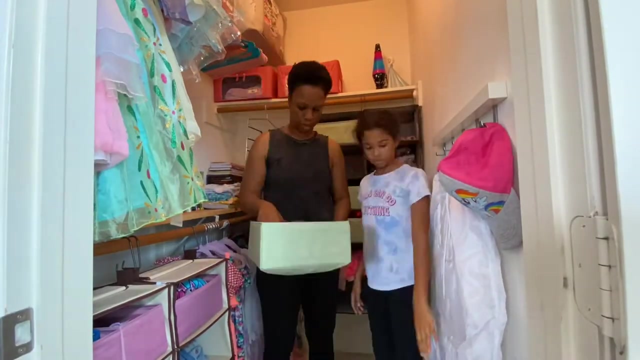 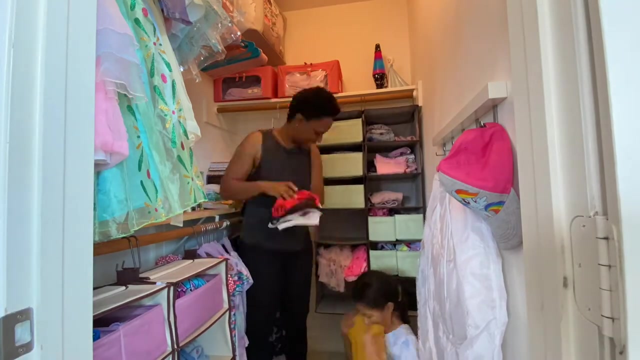 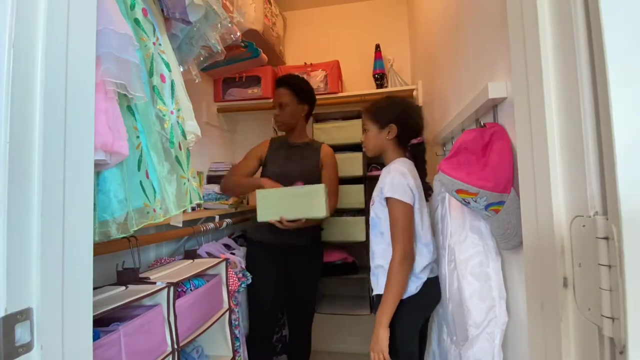 we cleared off the floor. these are things that we're going to give as gifts later on, some things going while off the in other places the tables mostly cleared. here's the trash pile. so the next thing we are going to do is go through the clothes and then we are going to take a look at some of the other things that we are going to take a look at. 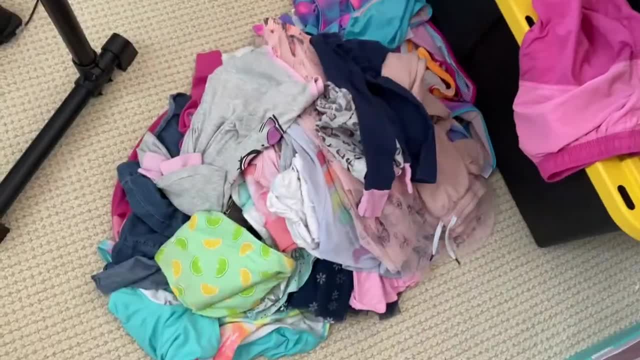 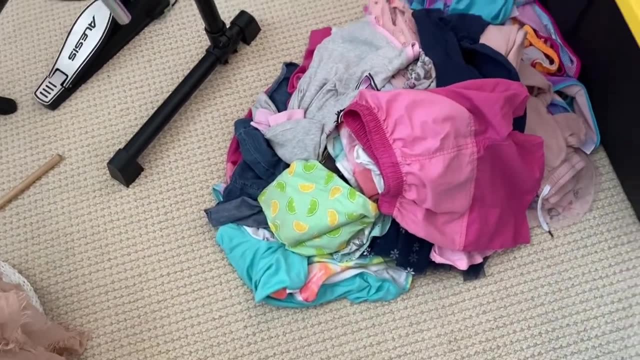 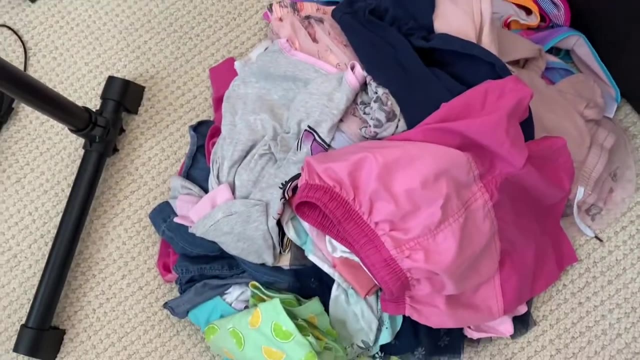 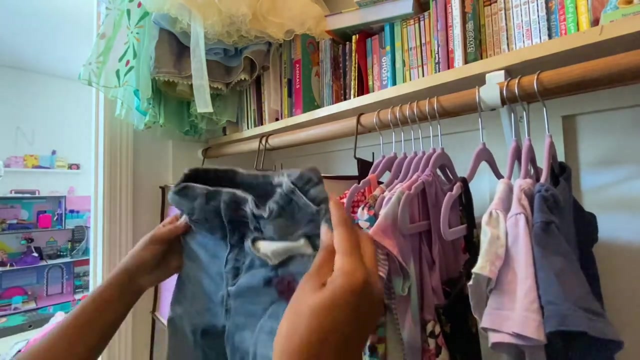 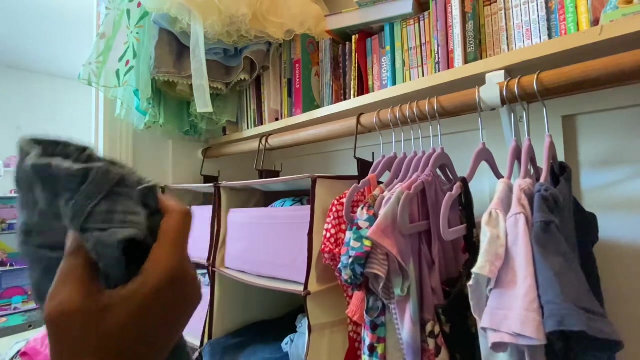 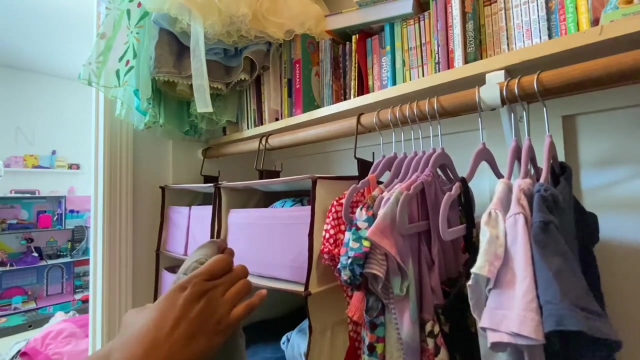 okay, these are all the clothes that we're decluttering from my oldest daughter's clothes, and we're gonna move on to the little ones first. let's go through your pants. okay, do you like these? these are nice pants. we'll keep those. what about these? oh, these are. these are 5t. can you fit these? can you try these on for me? okay? 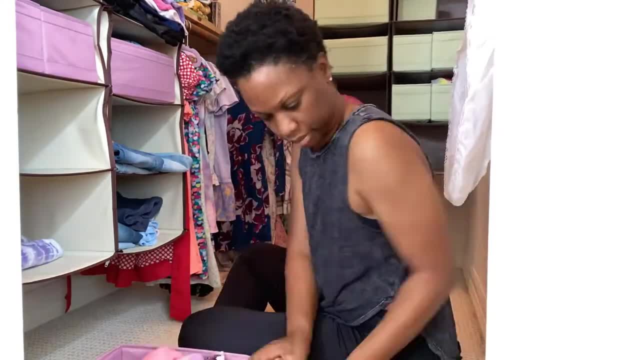 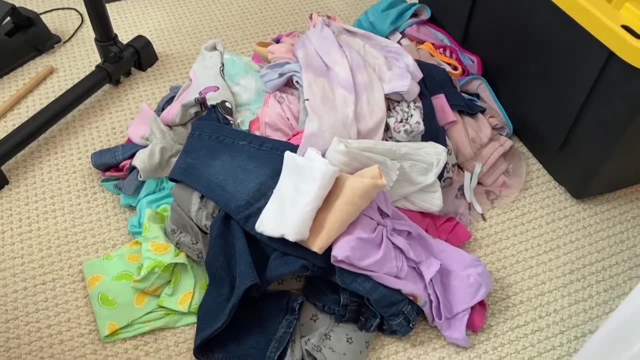 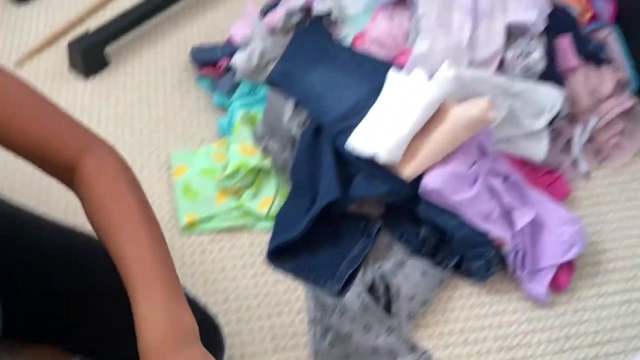 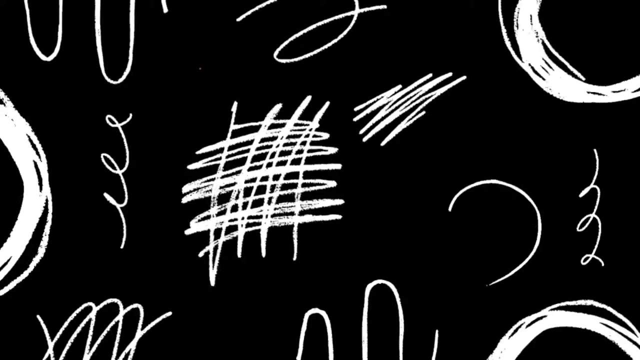 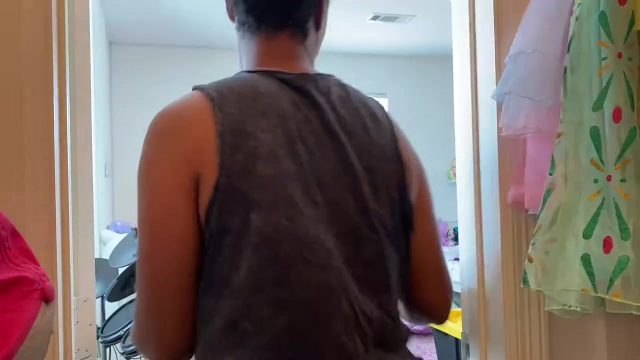 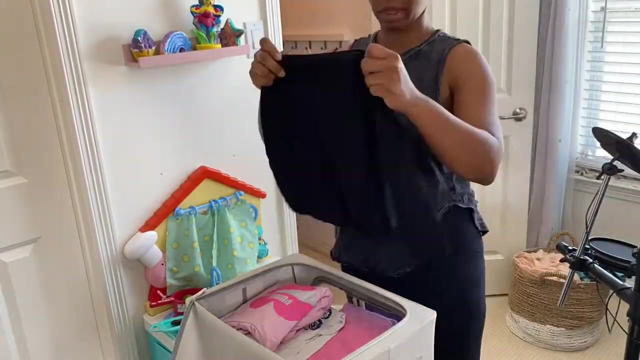 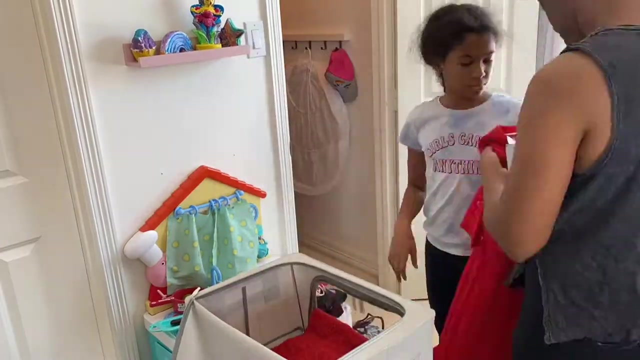 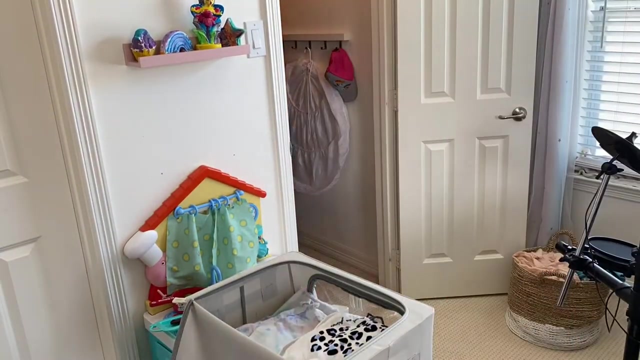 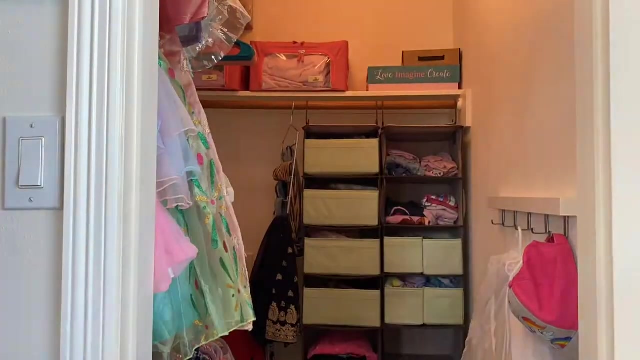 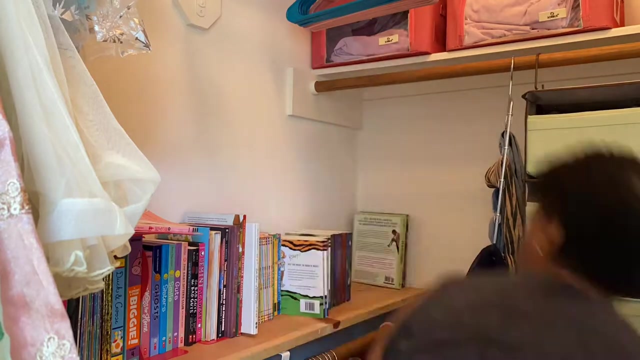 we're done, going through the girls hanging clothes and they're folded clothes and these are all the ones we are going to donate, and Nora has a garbage bag and she is going to put everything inside you. gg, g҉, ģ, ҕ, ҉, ҉, ҉, ҉, ҉. 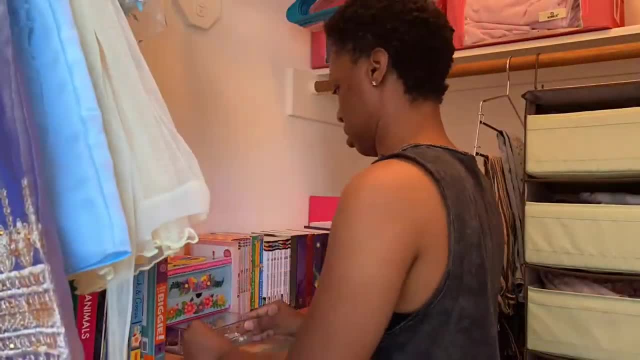 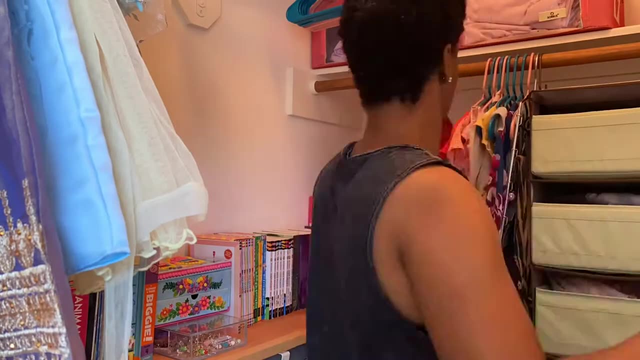 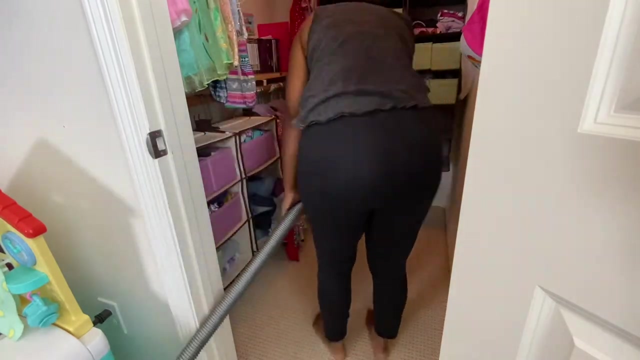 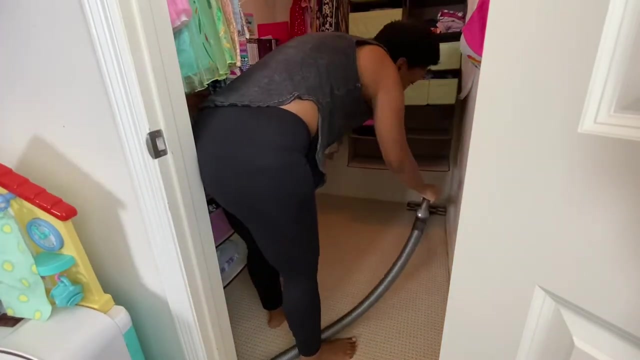 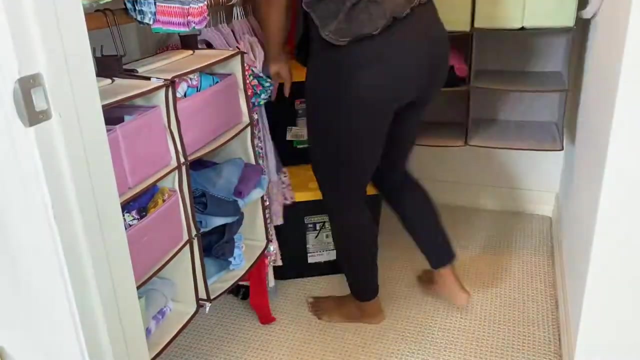 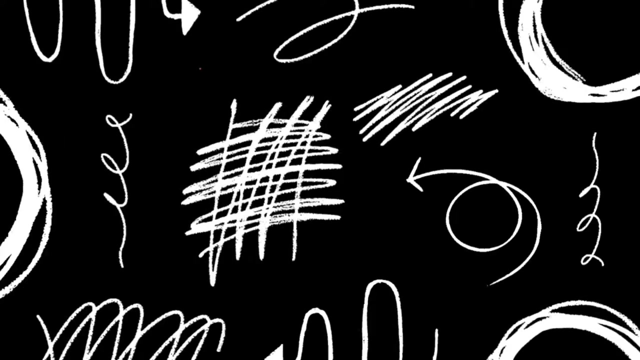 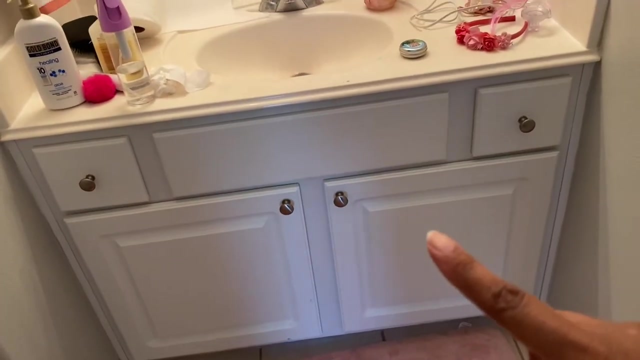 gg, fyan, gms, gks, gg, ggs, ggs, ggs know what that meant. I should have known better back then. If I could find a way, I would take back everything I want to change for you. Yeah, So next up is the bathroom, And the main thing I want to do is organize their vanity, their 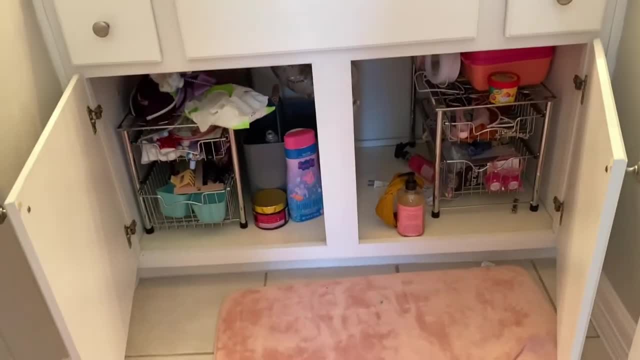 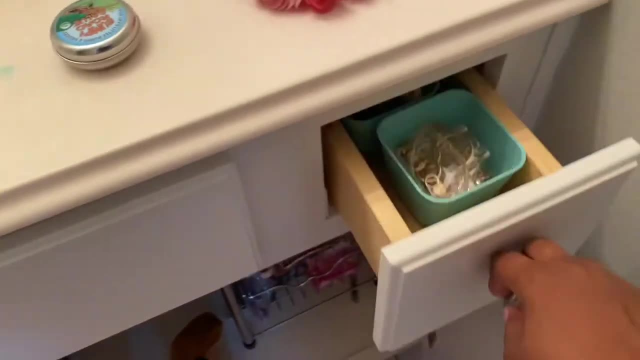 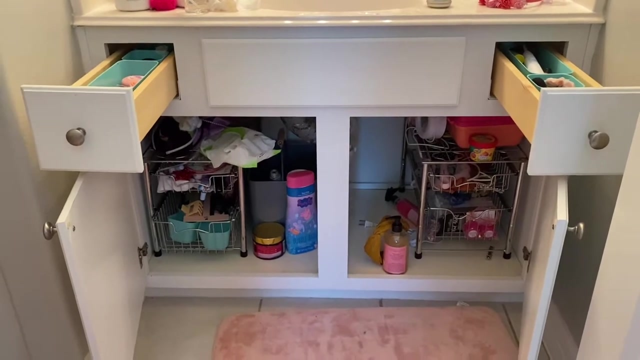 hair products. They have separate bins- This is my oldest daughter, youngest daughter- And then they each have a drawer. So I want to go through and organize these things, especially before school starts, Since when school starts, this is going to become a very, a very busy area. So 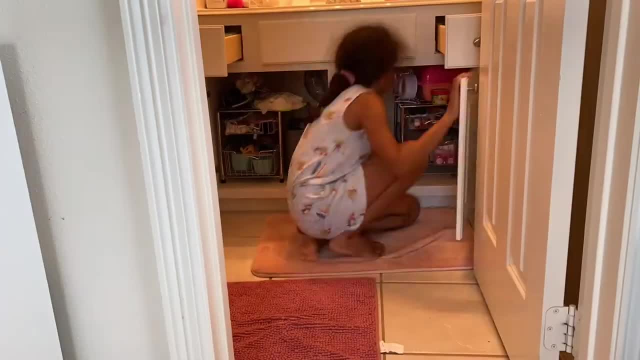 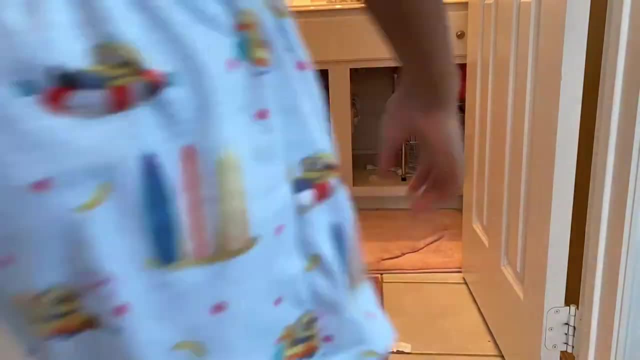 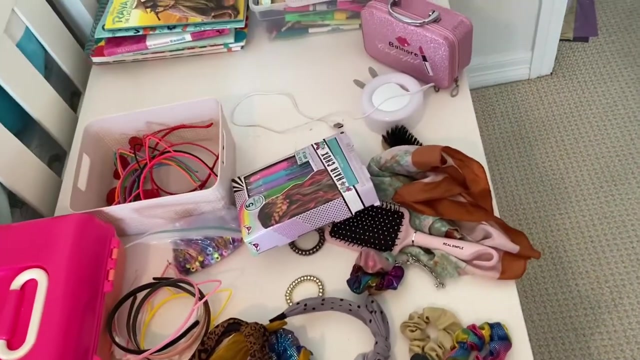 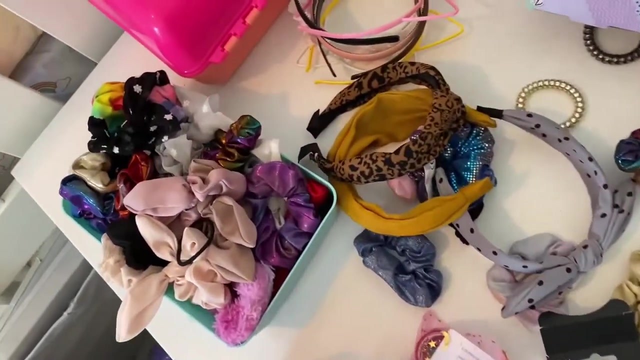 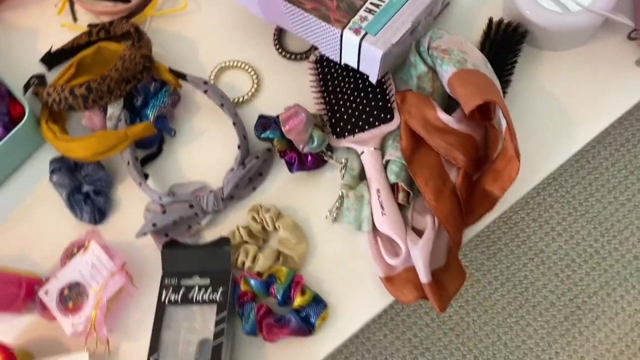 I'm going to take the big one and we're going to get started. So far, this is all the stuff from my eldest daughter's side of the bathroom. We've got tons of hair scrunchies and headbands and hair stuff. And let's get started, guys. 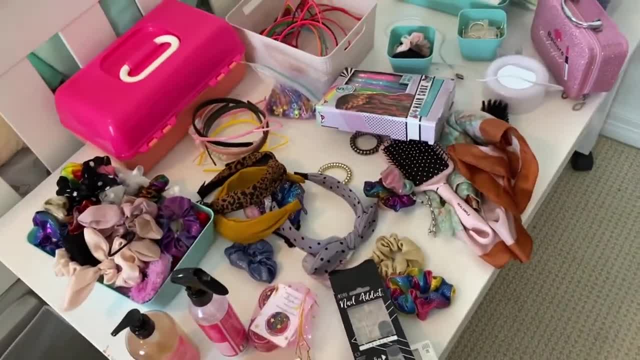 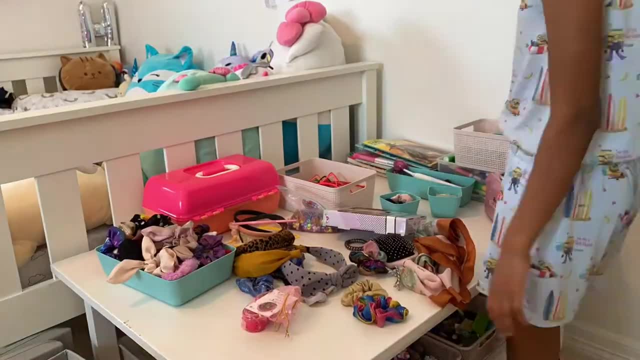 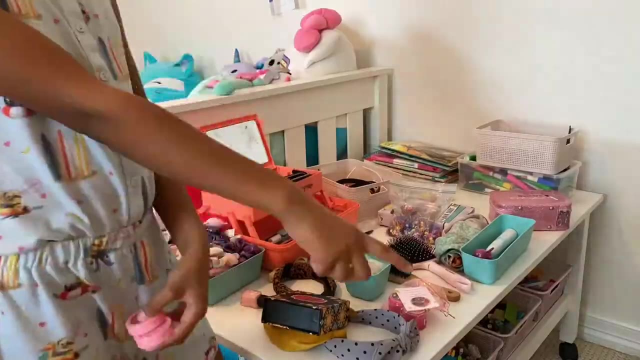 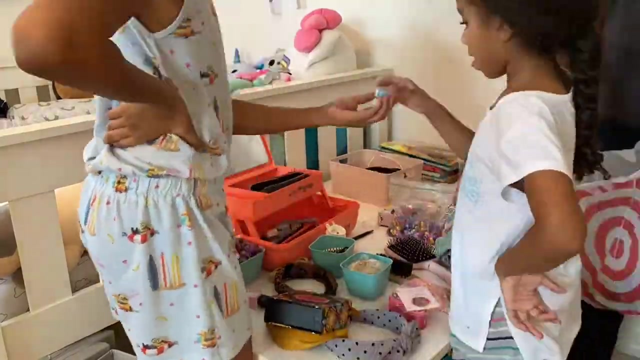 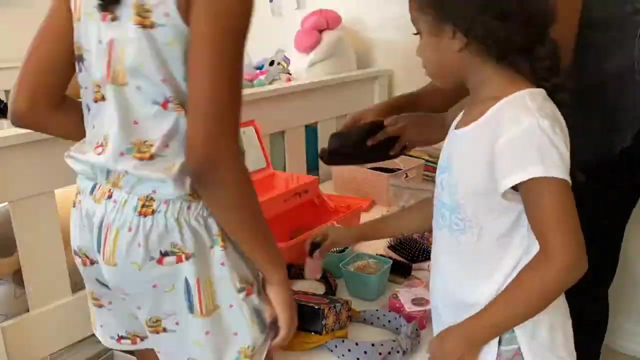 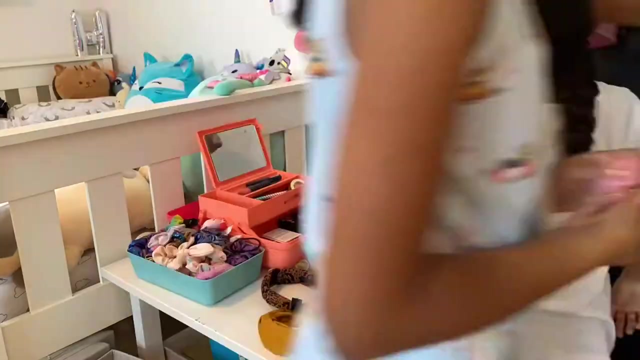 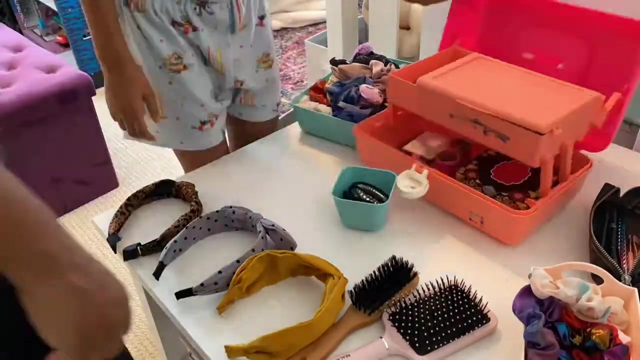 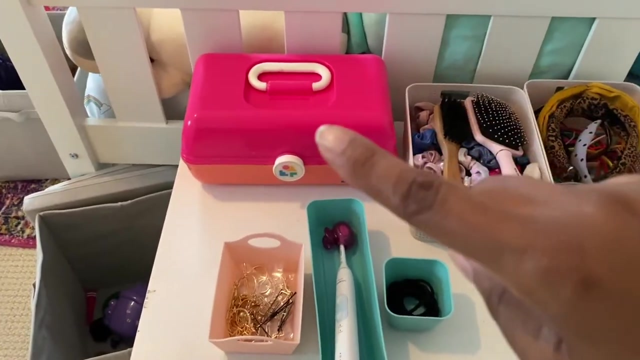 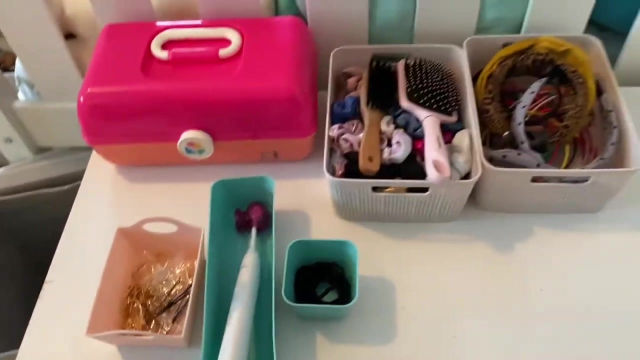 So we're going to to sort through this stuff, look at what we want to keep and then organize the rest, guys. so the big one has finished organizing her hair scrunchies and her, her makeup, her headbands, her hair barrettes and hair ties, so she's gonna put this back in the bathroom and 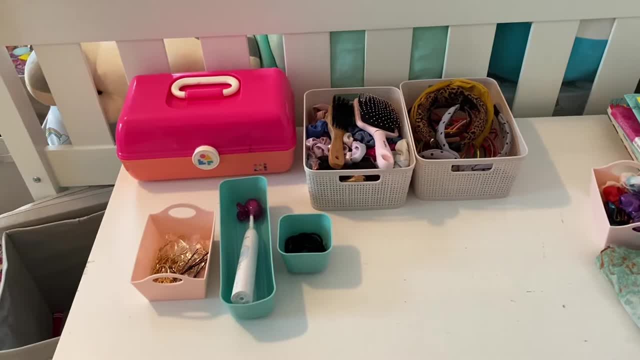 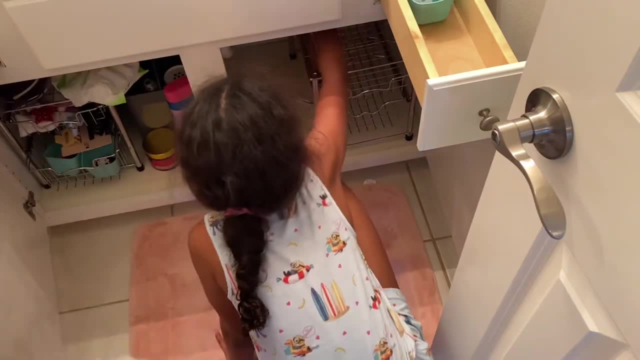 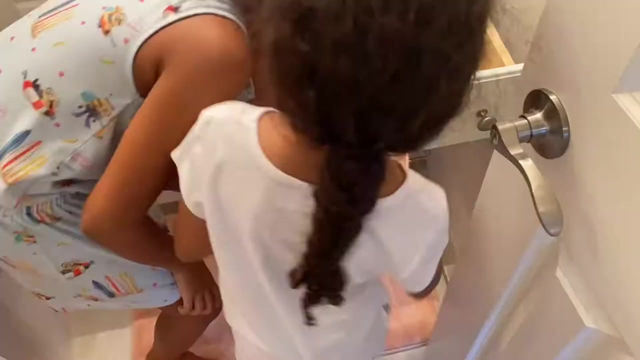 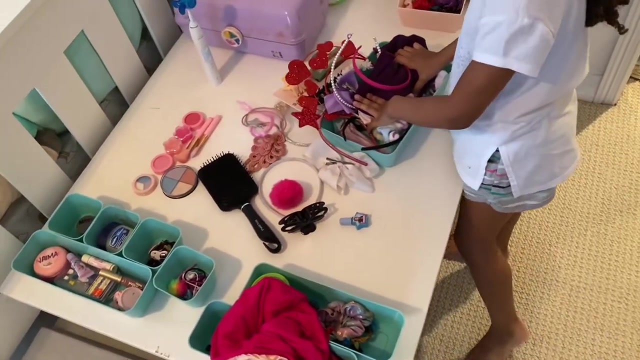 then we're gonna put this back in the bathroom, and then we're gonna put this back in the bathroom. we're gonna work on the little ones side, all right. so we've got the little ones things out here, so we're gonna go through and declutter. 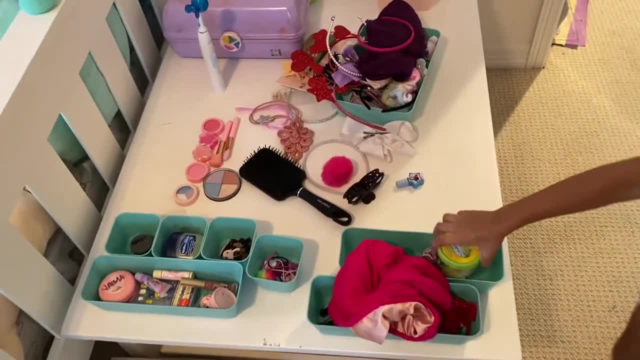 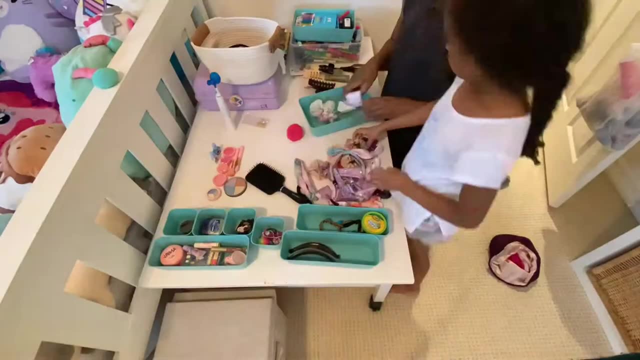 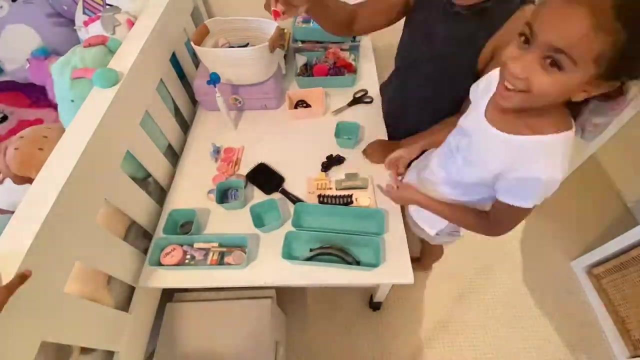 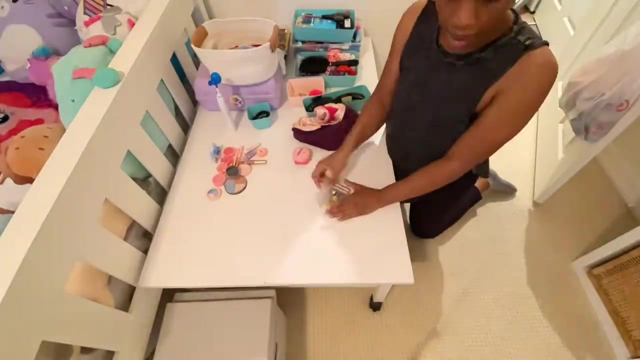 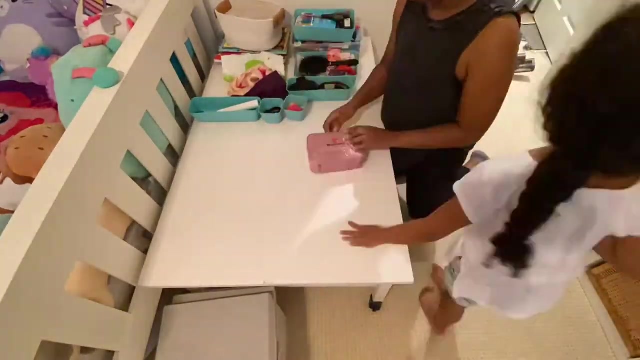 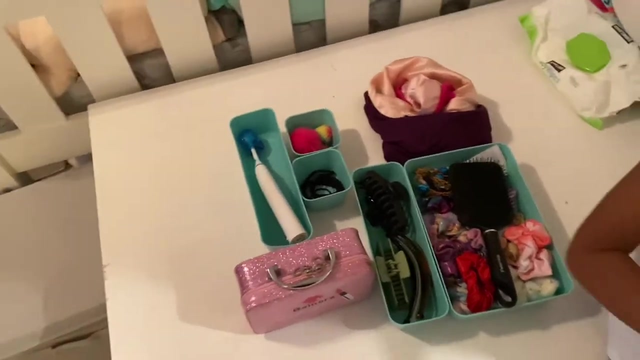 um and organize her, her things, all right. so we've got the little ones things out here, so we're gonna go through and declutter, all right. so we've got the little ones things out here, so we're gonna go through and declutter um the little ones: hair accessories and. 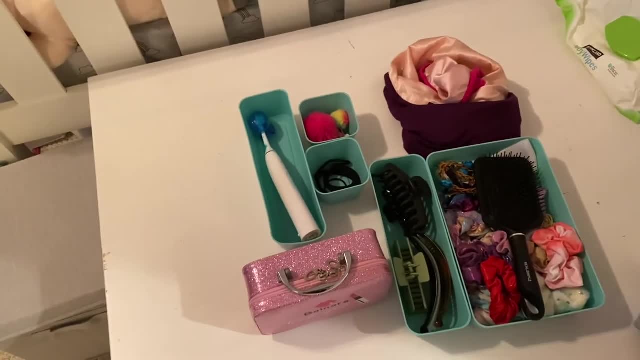 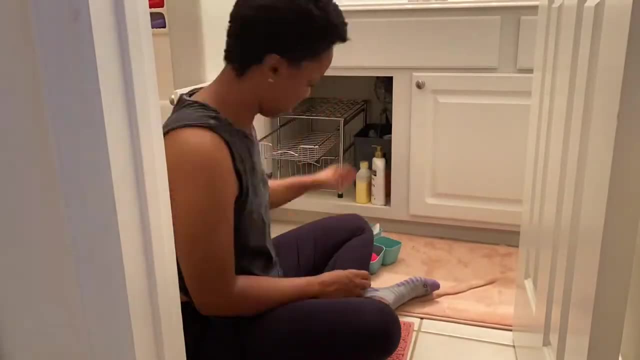 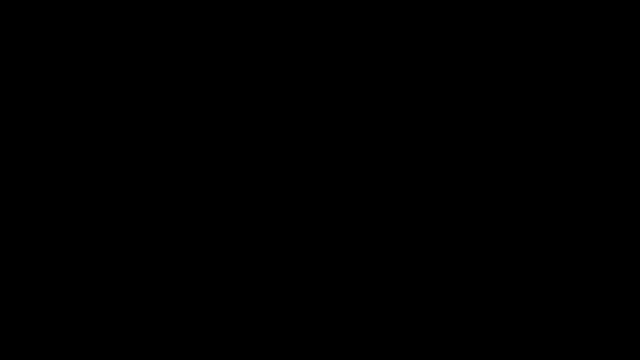 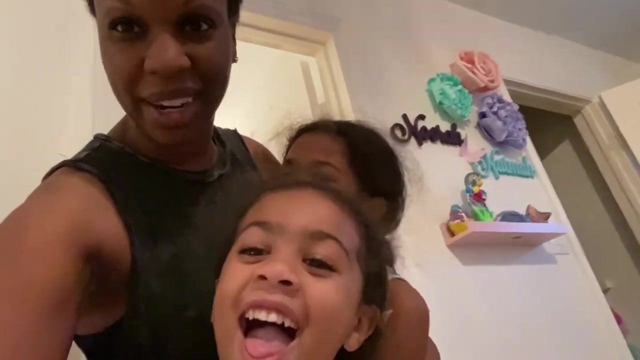 makeup, and so now we're gonna put her um stuff back on her side of the vanity. all right, guys. so we're gonna end this part of the video right here. guys, so we've got the little ones things out here, so we're gonna end this part of the video right here. 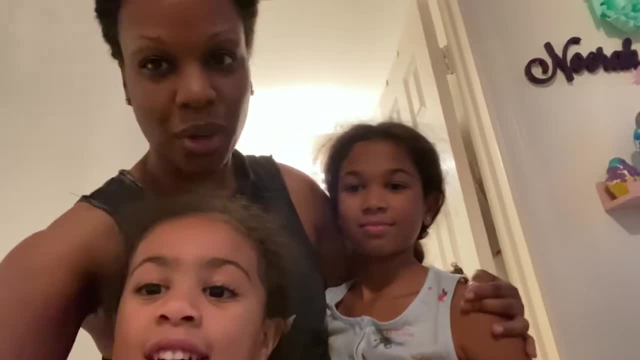 um, we decluttered the closet, we organized their closet, we decluttered and organized their bathroom vanity, um, and they'll clean their bathroom tomorrow because we are pooped after all that decluttering and organizing. so thanks for joining us. we'll see you guys again tomorrow when the bathroom is clean. all right, guys, bye, see you tomorrow. 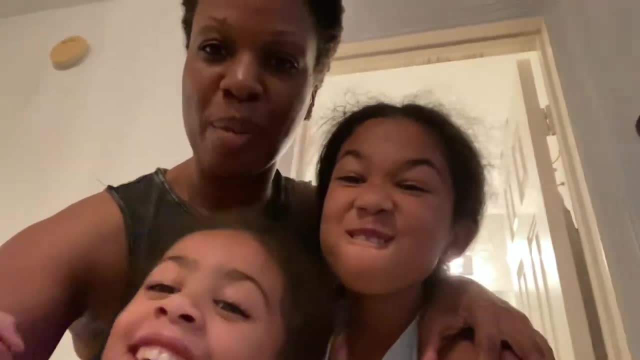 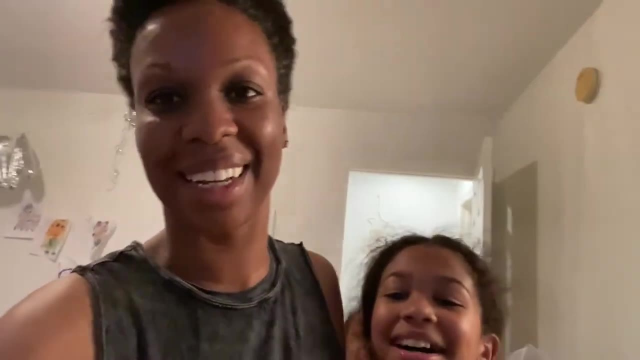 um, and they'll clean their bathroom tomorrow because we are pooped after all that decluttering and organizing. so thanks for joining us. we'll see you guys again tomorrow when the bathroom is clean. all right guys, bye, see you tomorrow. um, we decluttered the closet, we organized their closet, we decluttered and organized their bathroom vanity. um, and they'll clean their bathroom tomorrow because we are pooped after all that decluttering and organizing. so thanks for joining us. we'll see you guys again tomorrow when the bathroom is clean. all right guys, bye, see you tomorrow. um, we decluttered the closet, we organized their closet, we organized their closet, we organized their bathroom tomorrow, because we are pooped after all that decluttering and organizing. so thanks for joining us. we'll see you tomorrow when the bathroom is clean. all right, guys, bye. see you tomorrow. 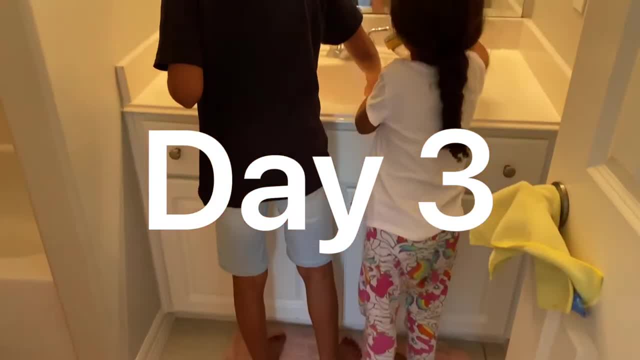 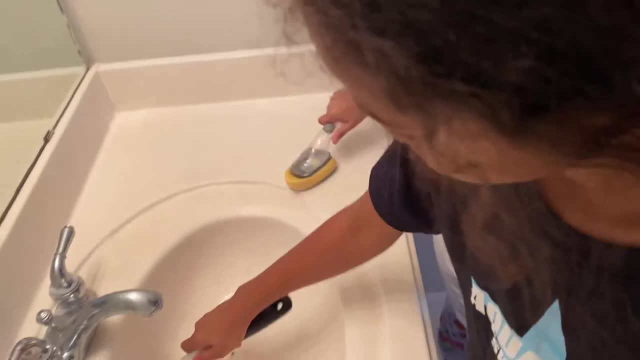 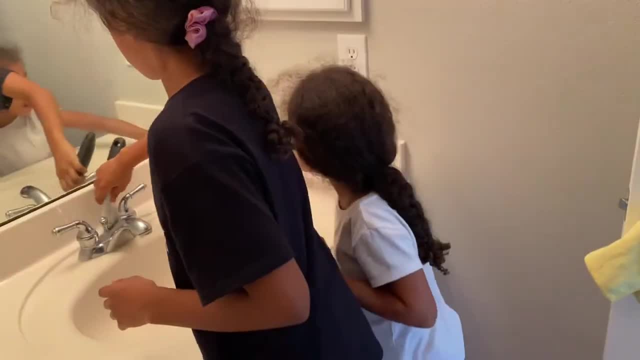 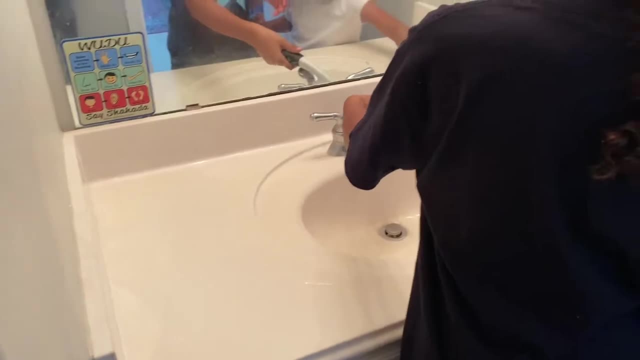 yeah, working together to clean, to clean their bathroom. so they've just got some scrub brushes and a little bit of Barkeeper's Friend. they are scrubbing their vanity. we're going to get our room vacuum accounting done. Should I use this to like scrub up here? 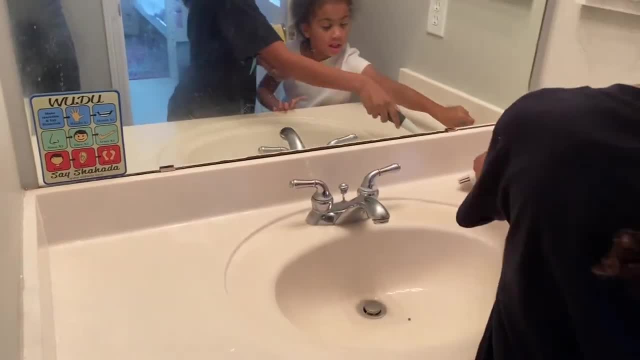 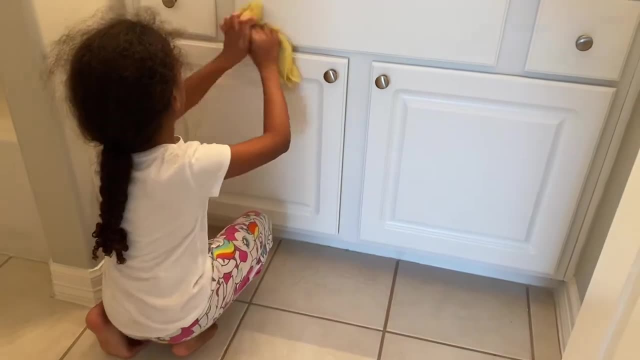 Um, you can, Or you can just use the microfiber towel, the e-cloth? Oh yeah, I could use that. Oh, at the end, I've been trying my best not to think about you, But you're stuck in my mind. 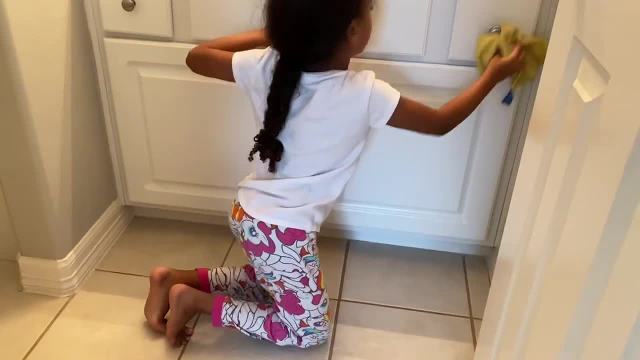 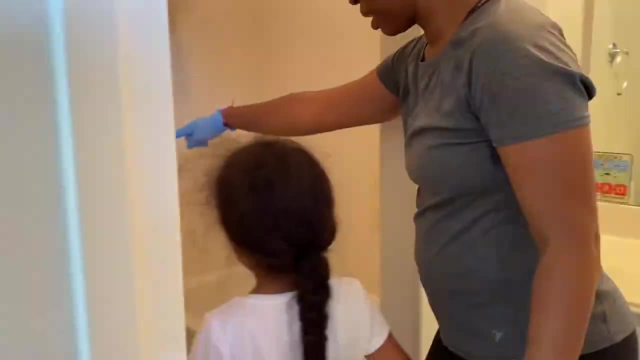 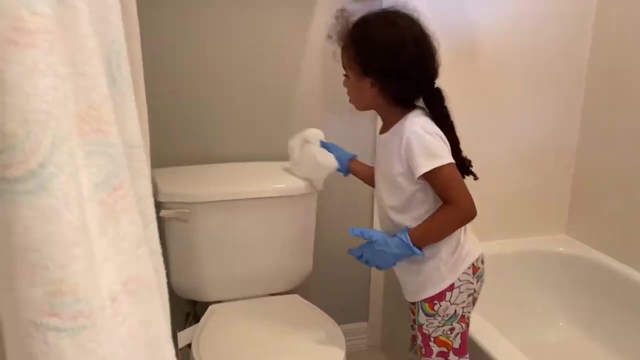 I've been hypnotized by you. All this suffering and pain got me feeling so blue, Because when it was us, I was never enough Girl. you got me thinking I was messed up, Pushing me down instead of pulling me up. 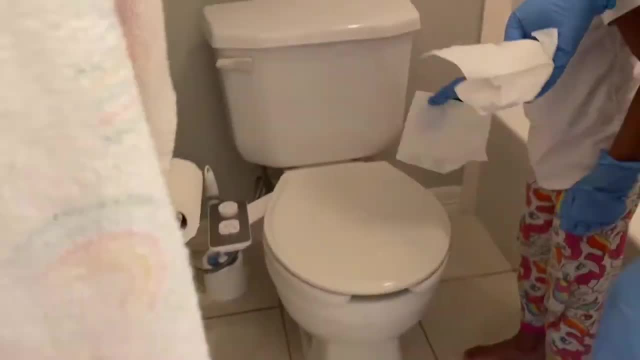 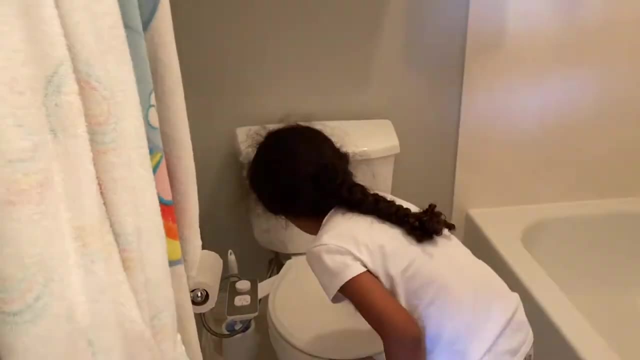 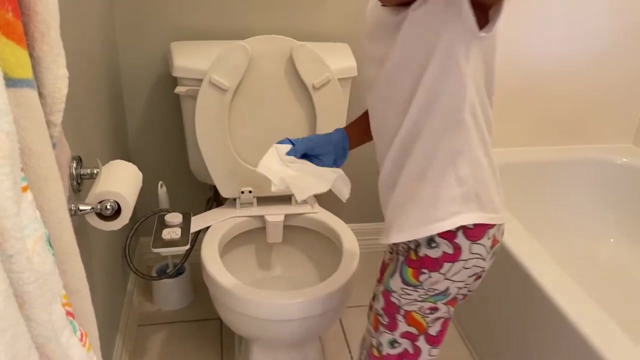 So tell me what I'm supposed to do. just to be all right, Girl, you got me thinking I was messed up. messed up, OK, good job. Hold on, I'm getting the garbage. Good job, I'm getting the garbage. 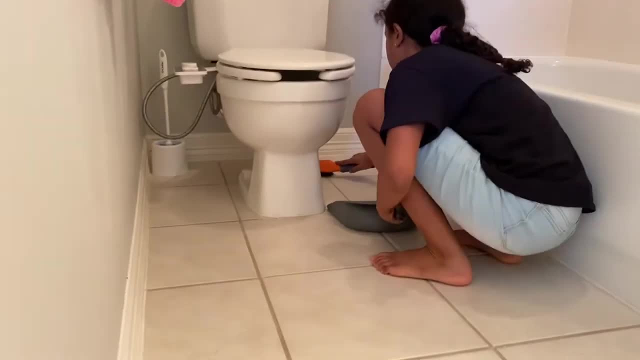 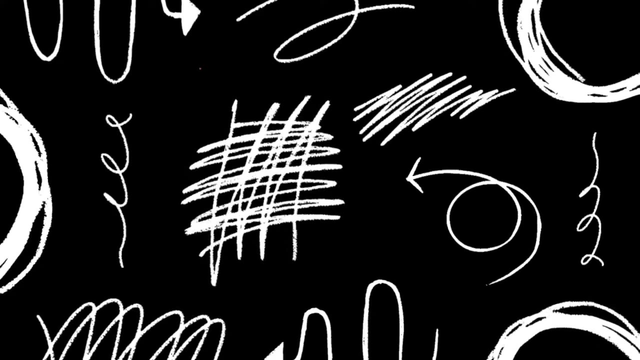 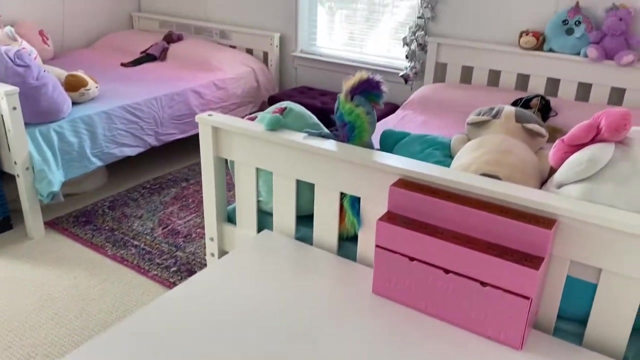 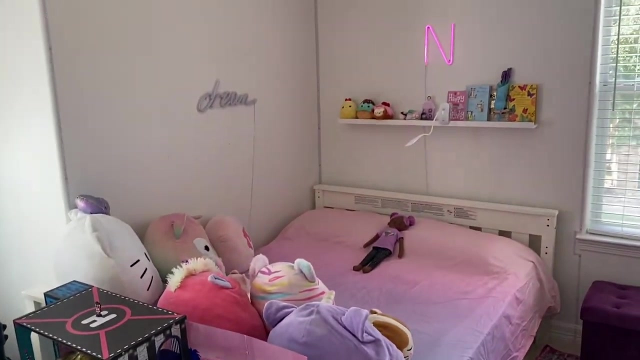 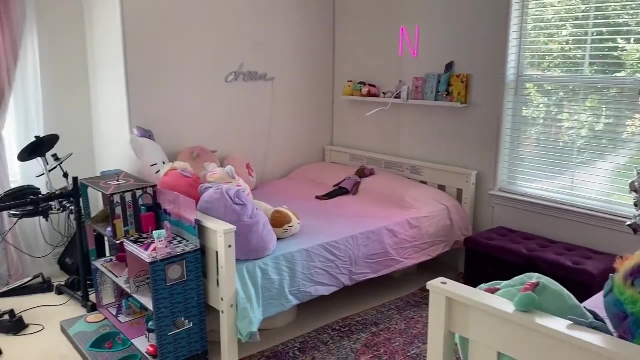 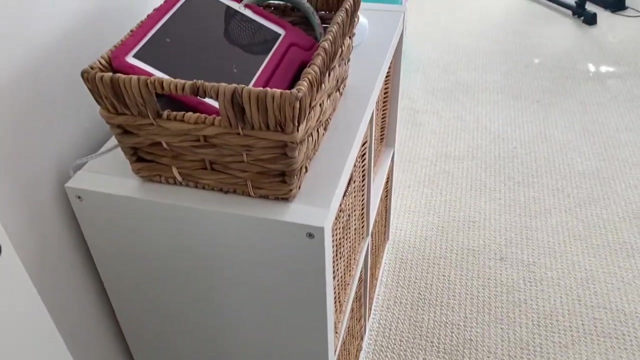 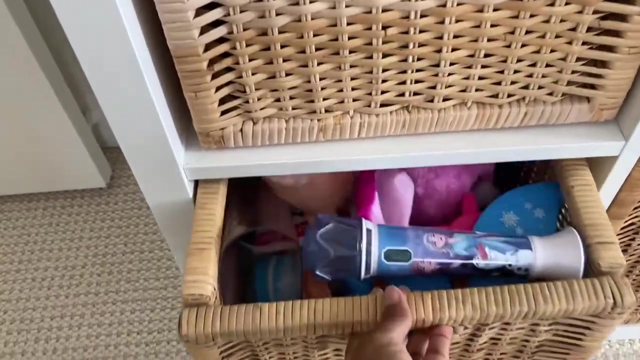 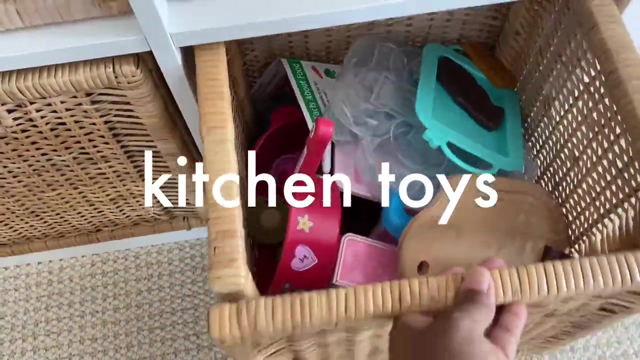 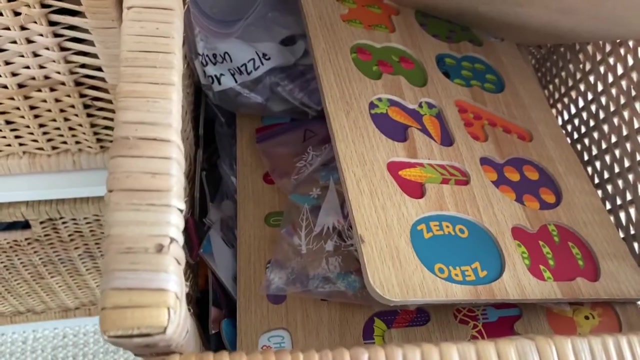 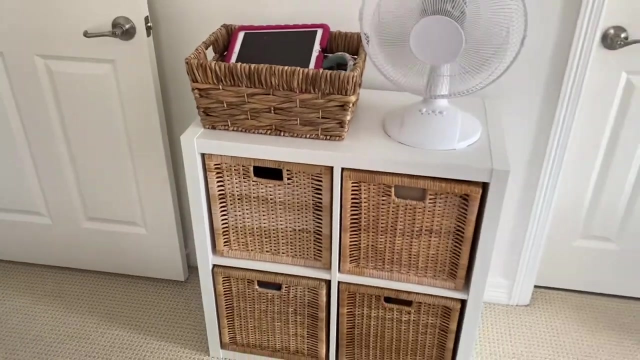 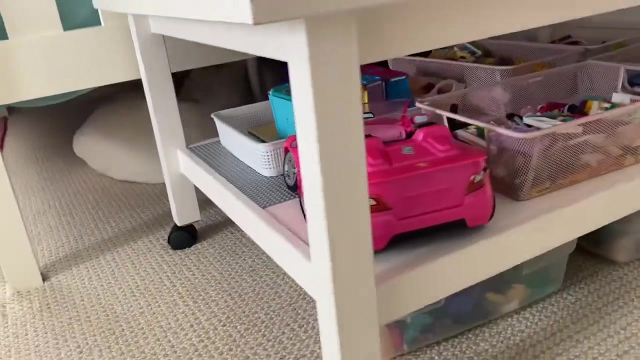 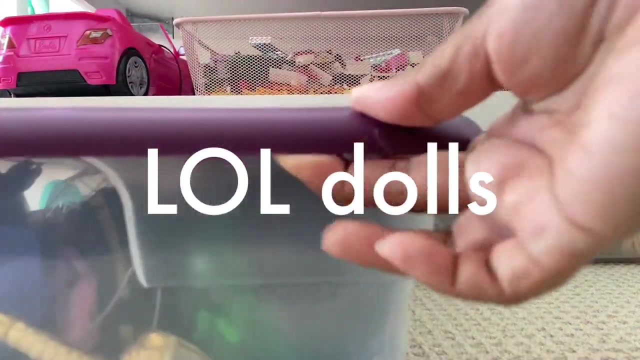 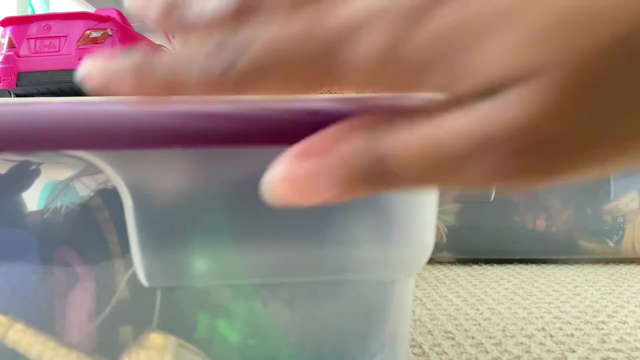 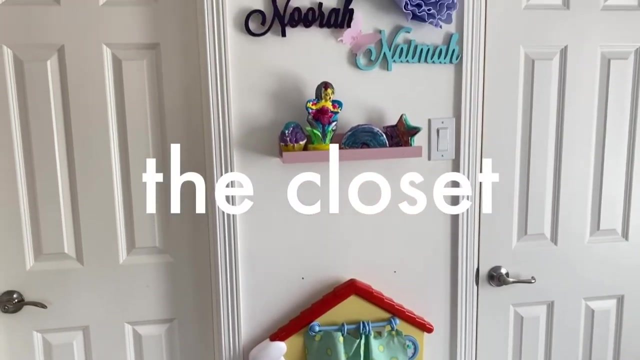 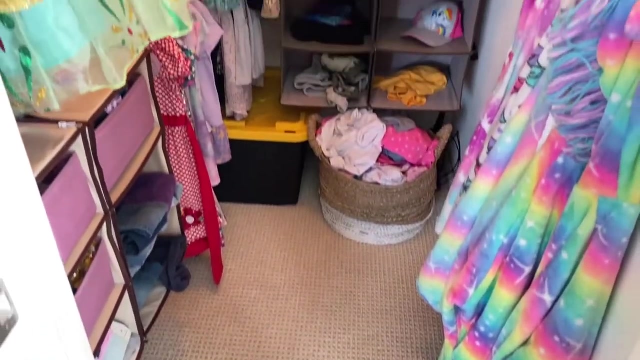 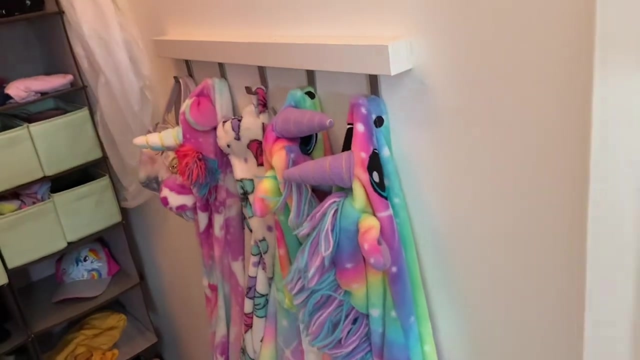 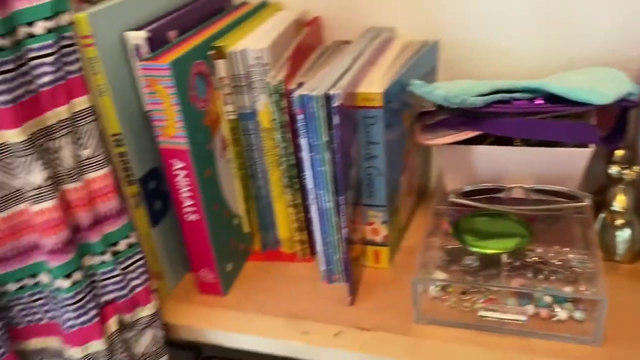 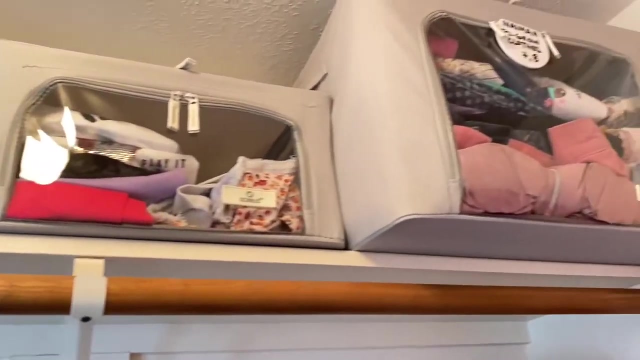 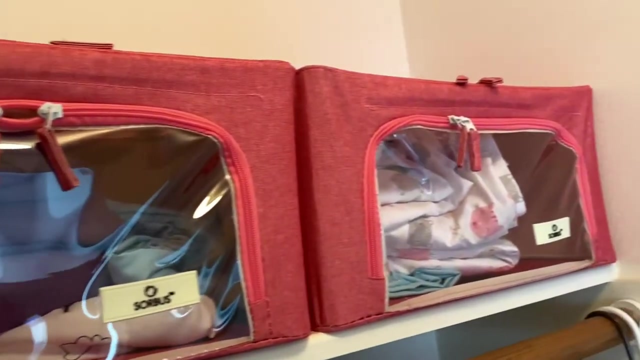 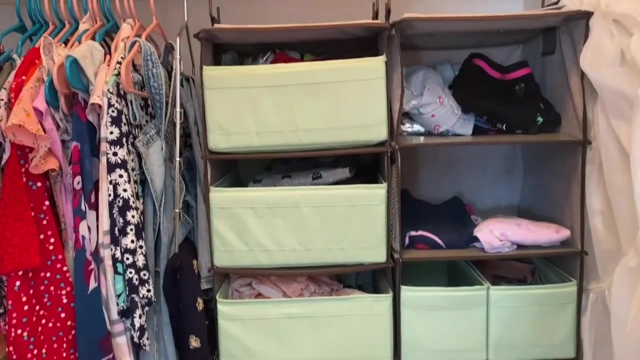 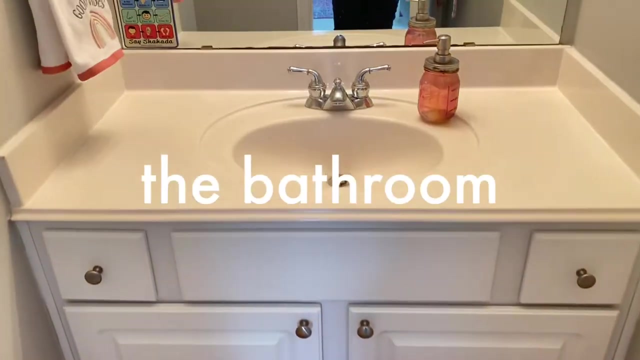 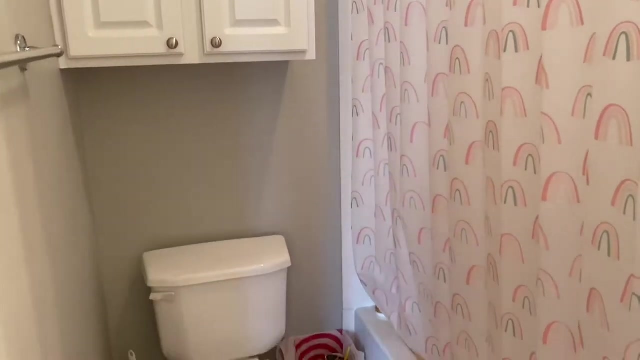 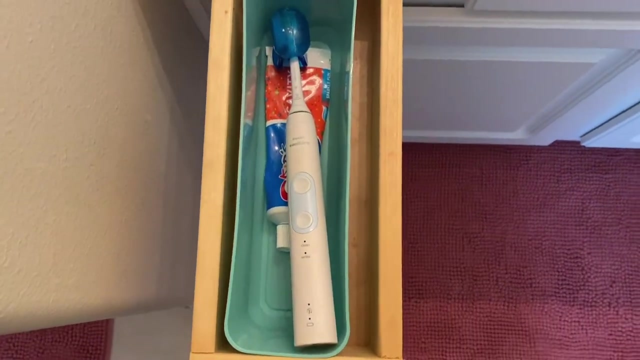 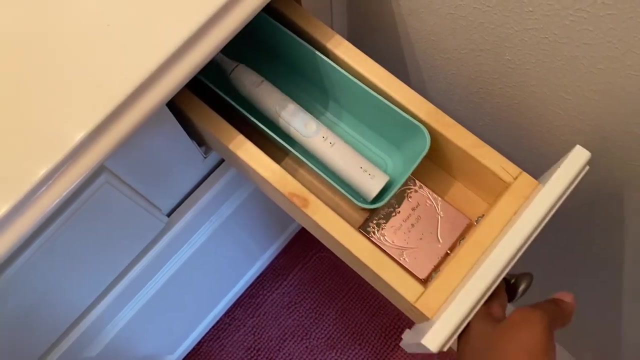 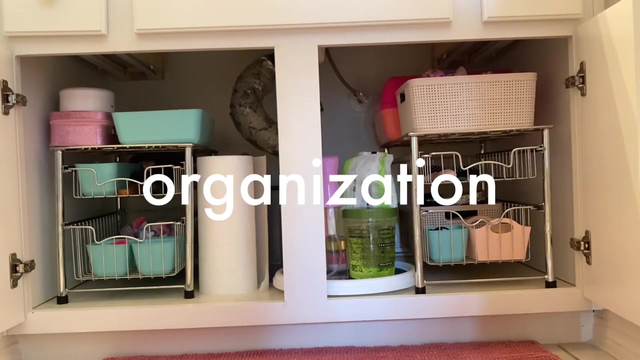 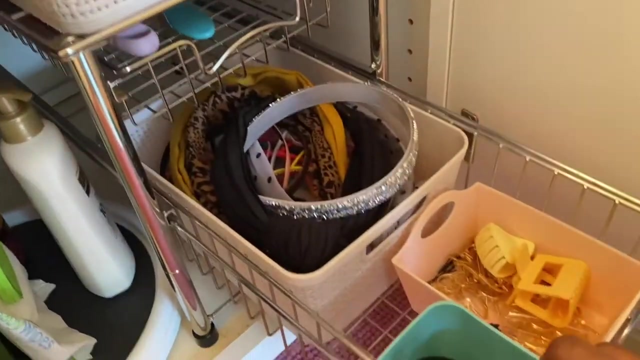 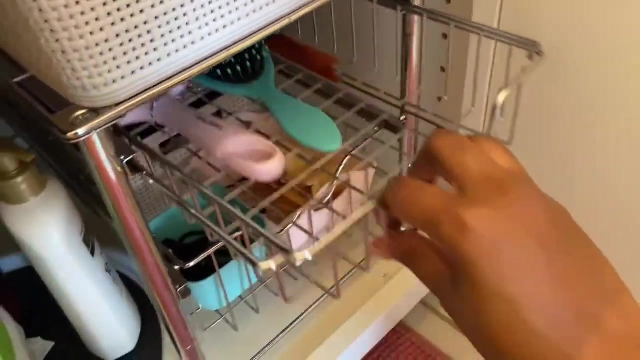 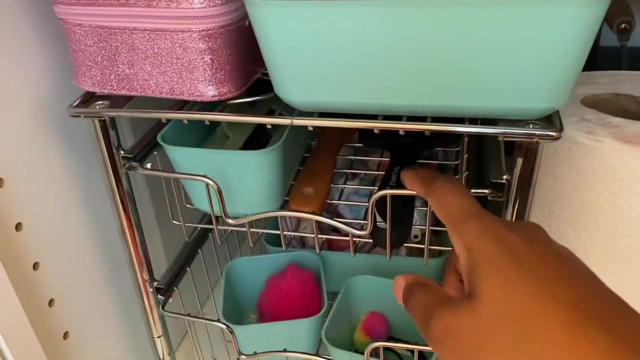 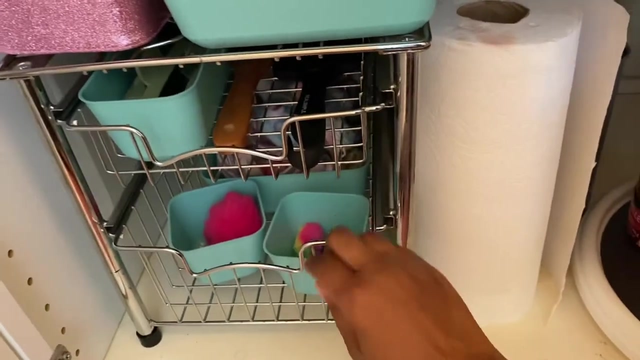 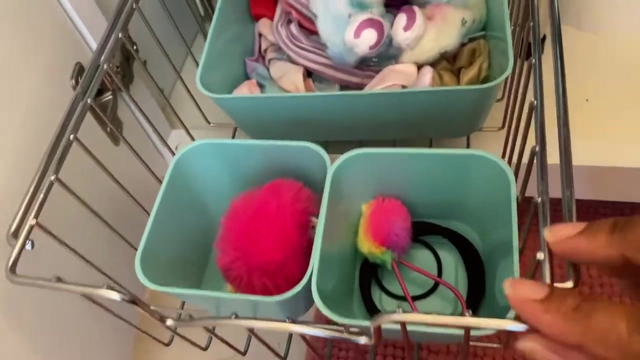 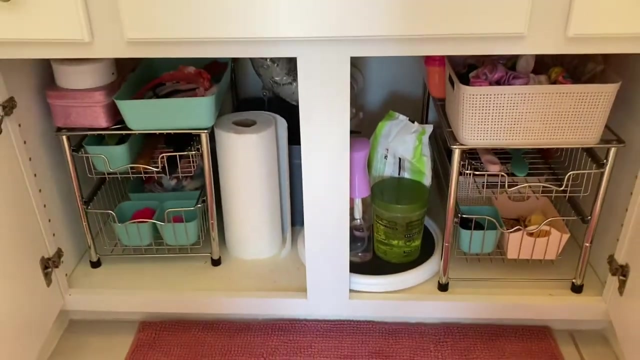 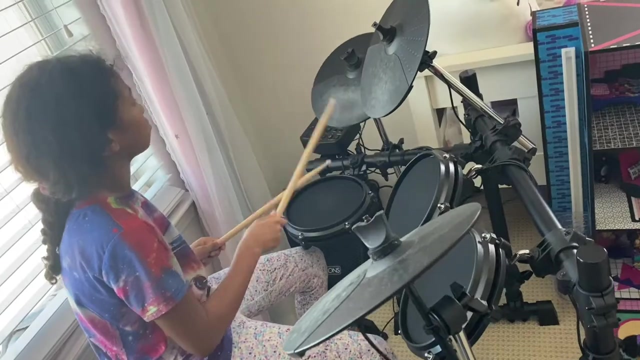 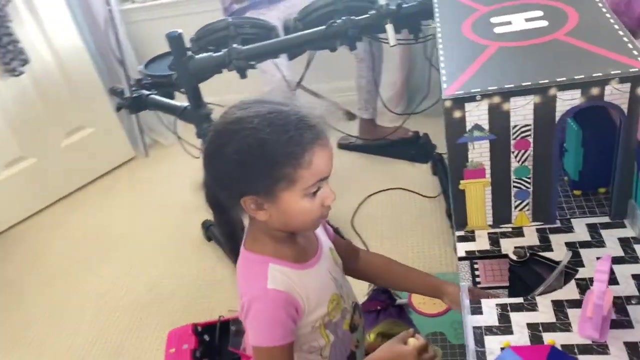